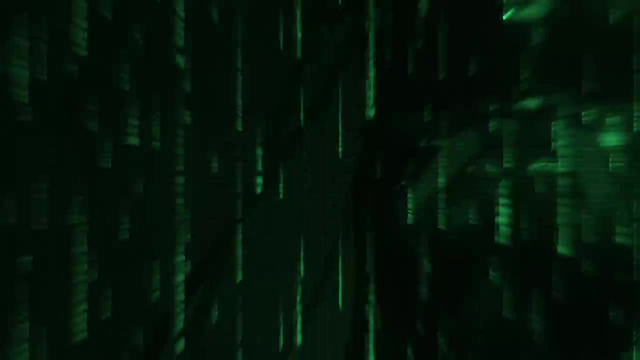 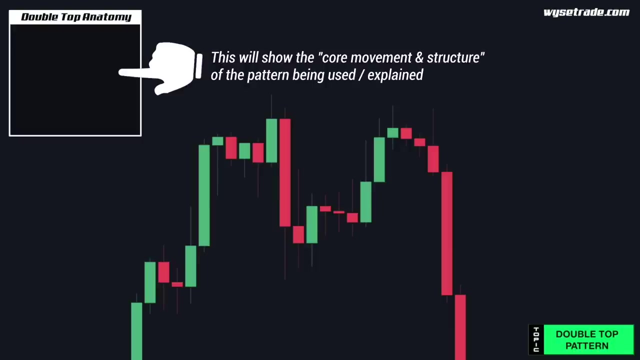 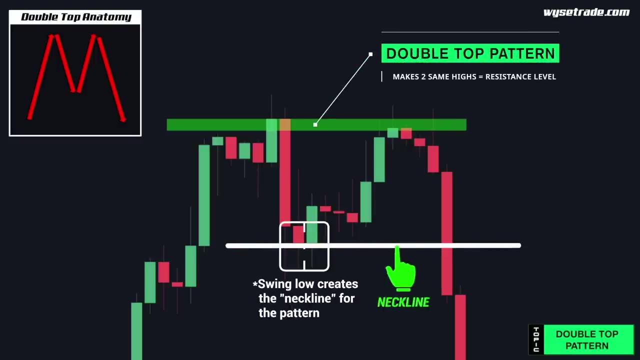 top- bottom pattern. Here is where we will be showing the anatomy of each pattern. So first you have your moving uptrend Price, then makes two same highs. The tops essentially make a resistance level, The swing low. here is what is called the neckline. 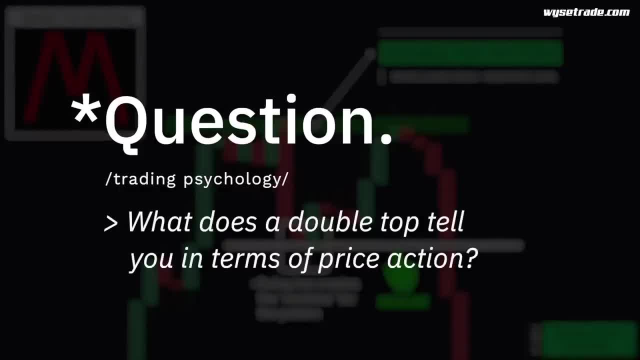 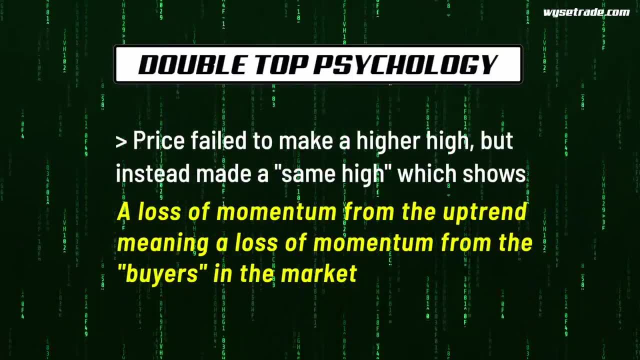 Now what does the double top tell you? from a price action standpoint, Price failed to make a higher high, but instead made a same high, which shows a loss of momentum from the uptrend, meaning a loss of momentum from the buyers in the market Now going the other way. 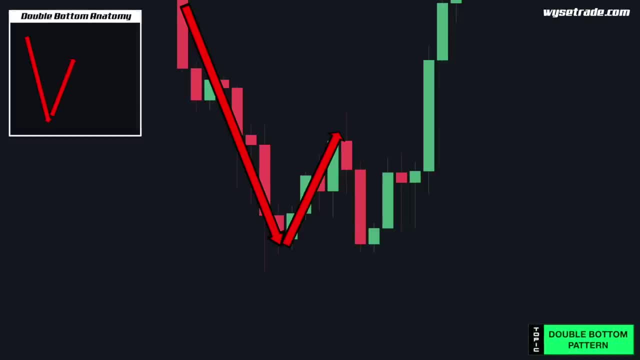 You first have your moving downtrend. Price then makes two same lows. The bottoms essentially make a support level. This swing high here forms the neckline. Now what does the double bottom tell you from a price action standpoint? Price then makes two same lows, The bottoms essentially 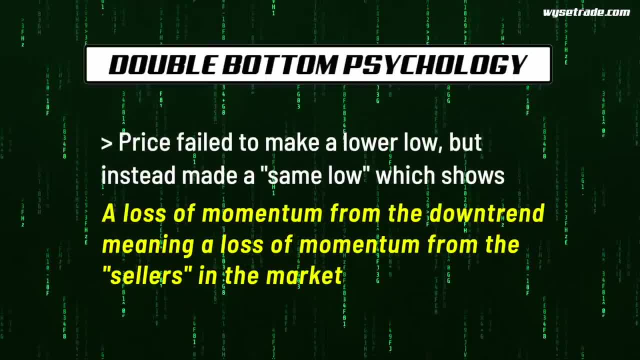 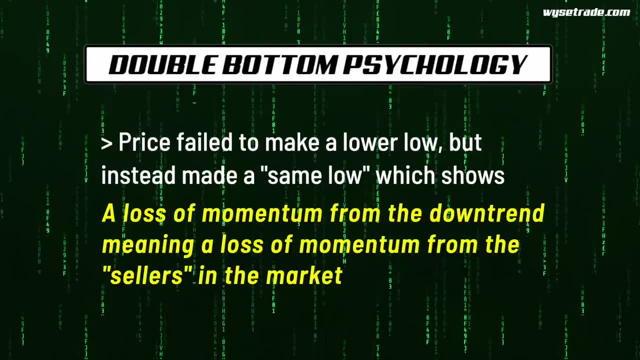 make a resistance level. This swing high here forms the neckline. Now what does the double top tell you in terms of price action? Price failed to make a lower low, but instead made a same low, which shows a loss of momentum from the downtrend, meaning a loss of momentum from the sellers in the market. 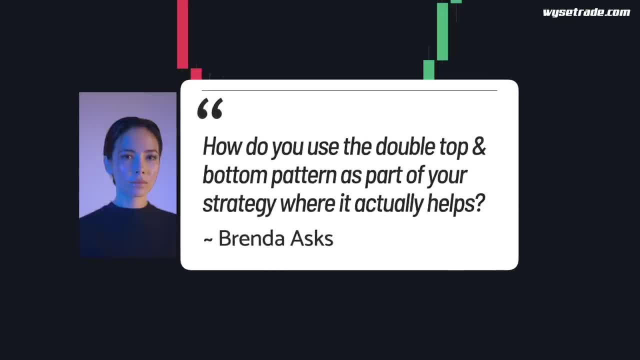 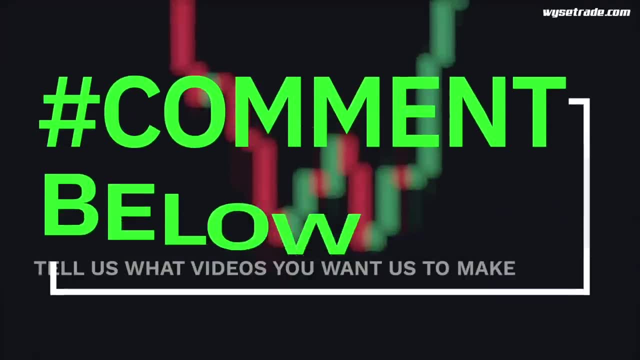 So this then brings us to our next question, which is: how do we use the double top and double bottom pattern as part of our overall strategy? Also, right now, go to the comments section below and tell us exactly what topics and questions you want us to cover. Also right now, go to the comments. 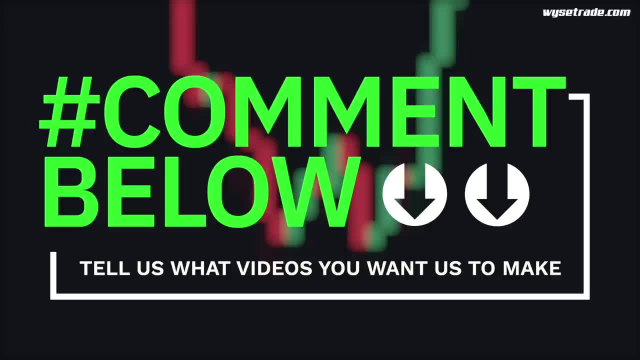 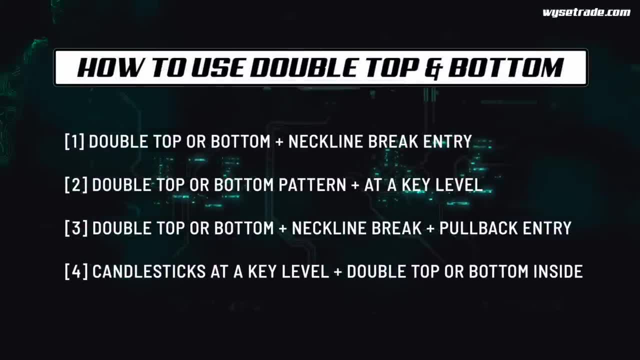 section below and tell us exactly what topics and questions you want us to cover, As we always look at the comments to decide what to create next. Now, these are the four core variations to using the double top and double bottom pattern. Let's start with the first, which is the neckline break. 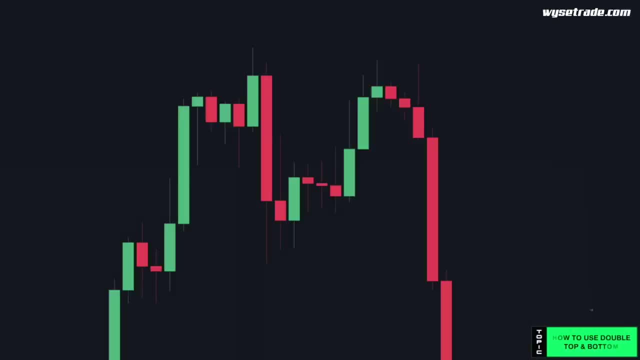 entry. So you first have your double top pattern that forms Neckline here because of the recent swing low. Now, once price breaks the neckline it makes a loss of momentum from the buyers in the market. Now, once price breaks the neckline and makes a lower low, you would take a breakout entry. 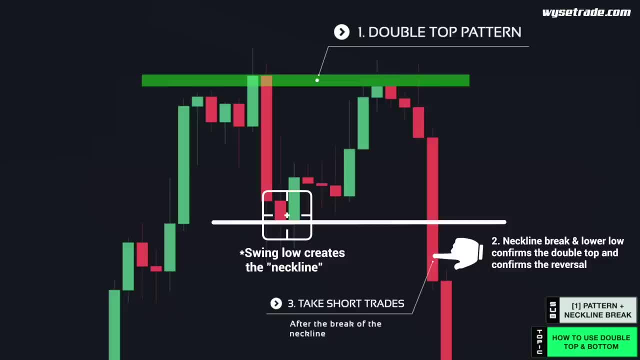 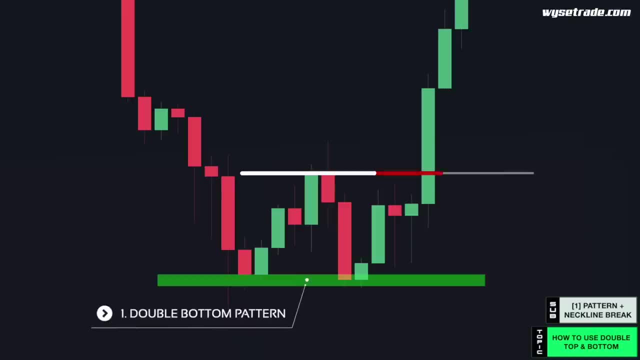 short as the reversal and trend change is now confirmed. Going the other way, you first have your double bottom pattern that forms Neckline here because of the recent swing high. Now, once price breaks the neckline and makes a higher high, you would take a breakout entry long as the 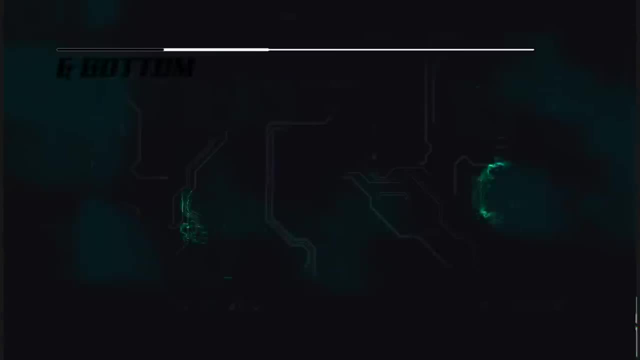 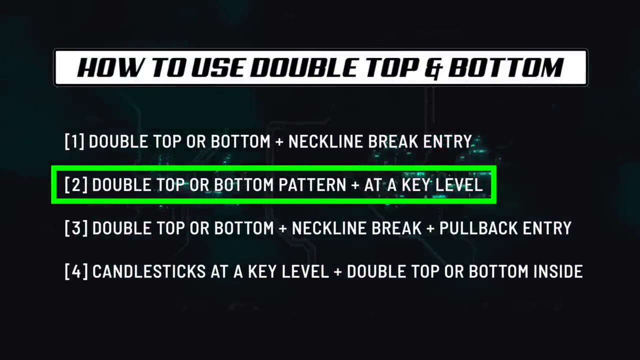 reversal and trend change is now confirmed. So moving on to the second variation, a double top or double bottom pattern forming a loss of momentum from the buyers in the market. Now, once price breaks the neckline and makes a higher high, you would take a breakout entry long as the reversal and trend change is now confirmed. Going the other way, you would take a breakout entry short, as the reversal and trend change is now confirmed. Going the other way, you would take a breakout entry long, as the reversal and trend change is now confirmed. Now, this is an entry that 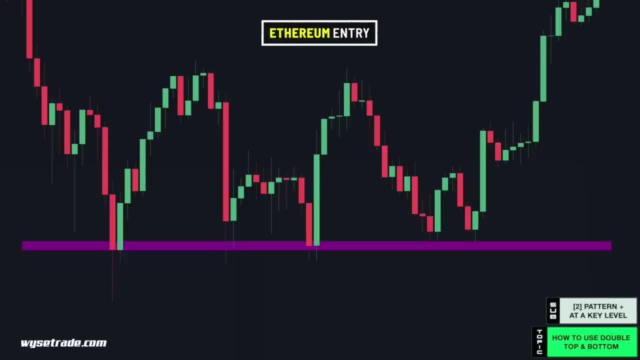 occurred on Ethereum and one that many of our members took. So you first need to identify a key level, which you have through these three reversal points. As price comes back down, it creates a double bottom pattern at the support level. So again to confirm the reversal. 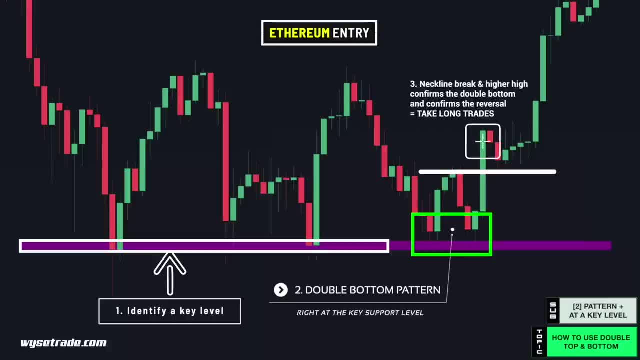 neckline placed at the recent swing high and once price breaks through the neckline and makes a higher high, your trend change from a downtrend to an uptrend is confirmed and you would then take trade entries long through the lower intraday timeframes. 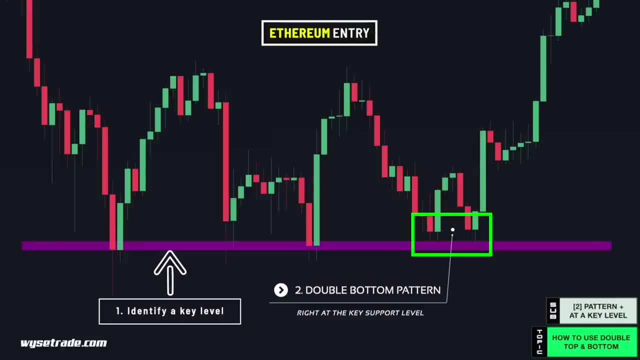 Now to point something out. there was another trend change confirmation you could have used, which was placing a trend line like this, connecting the swing highs, and again waiting for the breakthrough, before looking for trade entries long Now going the other way. 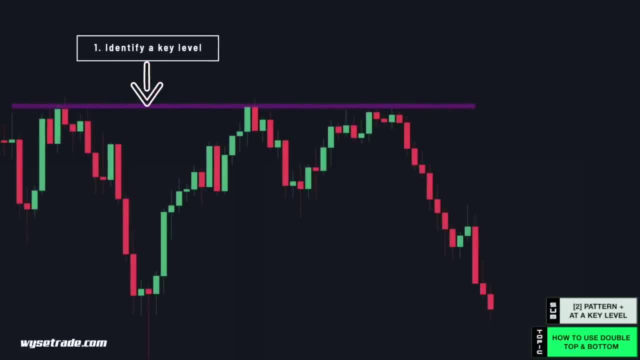 Again, you first need to identify a key level which you have through this reversal point here, giving you your resistance level. As price comes back down it creates a double top pattern right at the resistance level. So again, to confirm the double top reversal neckline placed at the recent swing low here. and once price breaks through the 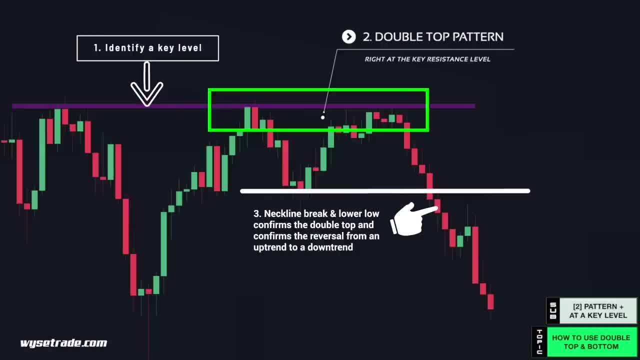 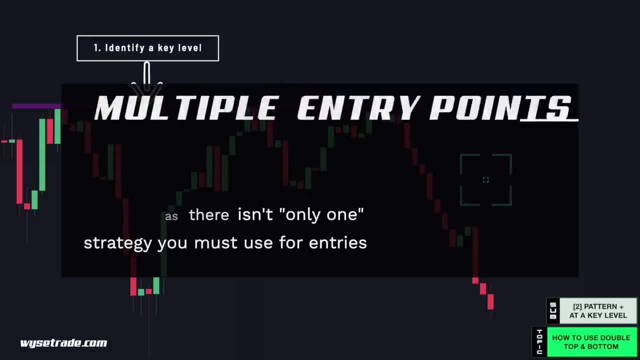 neckline and makes a lower low, your trend change from an uptrend to a downtrend is confirmed and you would then take trade entries short through the lower intraday timeframes. This is also a very good example of the many different opportunities there are to enter trades. 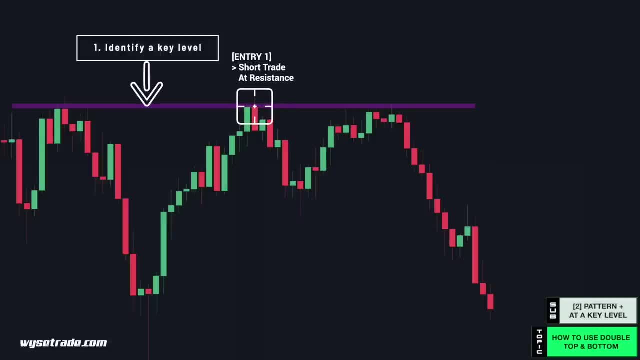 Some would have entered short right at this point here. Are there any other opportunities to enter trades? Others would have entered short right at this point here, where pattern traders wouldn't enter until the double top pattern formed and then the break of neckline. here All are correct. There are. 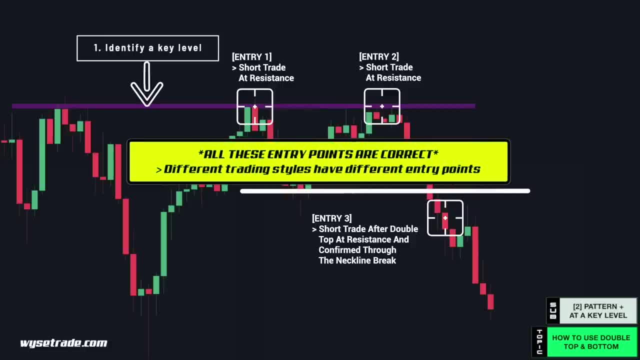 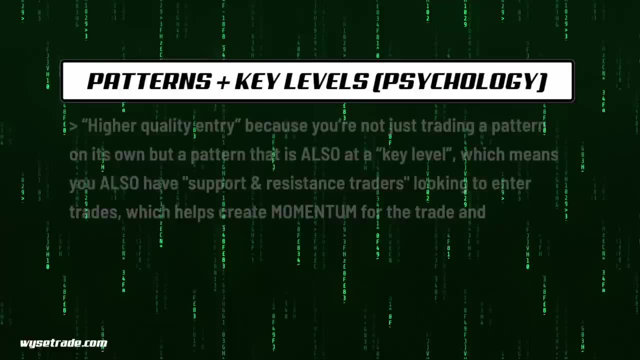 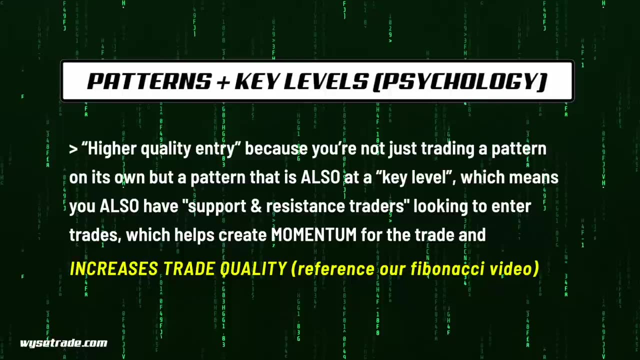 multiple different ways to enter trades, based on your style. So what does the double top or double bottom pattern at a key level tell you? from a price action standpoint, This kind of entry is of higher quality because you're not just trading a pattern on its own, but a pattern that is also 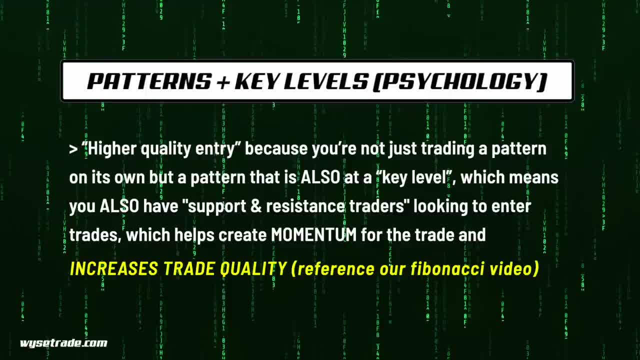 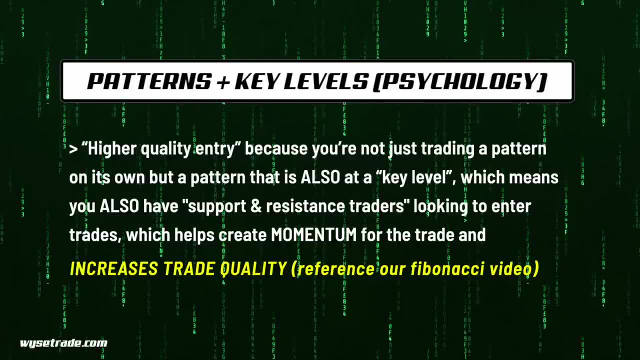 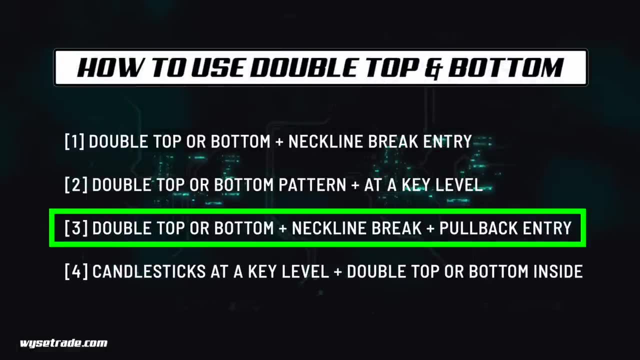 at a key level, Which means you also have support and resistance traders looking to enter, along with pattern traders, which helps create momentum for the trade and increases trade quality. So, moving on to the third variation, a double top or double bottom pattern, but instead of taking 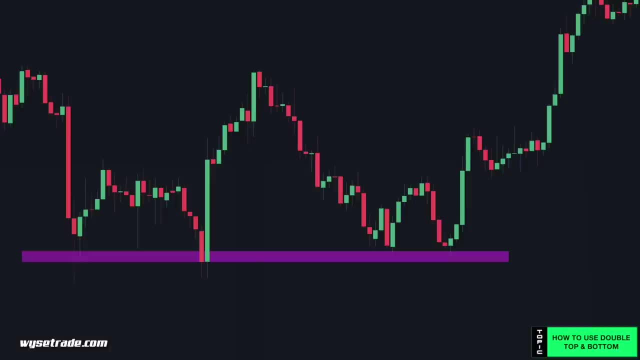 the breakout entry waiting for a pullback entry. So back to the Ethereum example we just covered. You had your double bottom pattern neckline break, but instead of taking the breakout entry, there was a second long entry on the pullback to the new support level. This is actually. 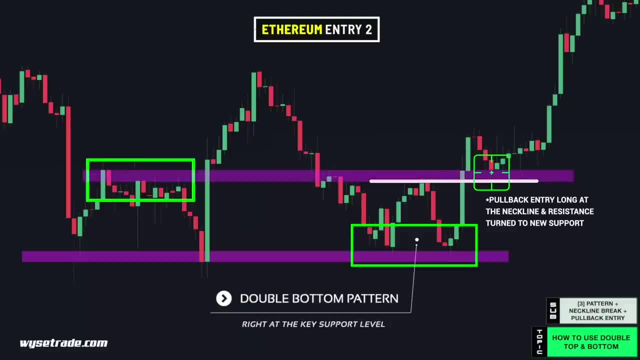 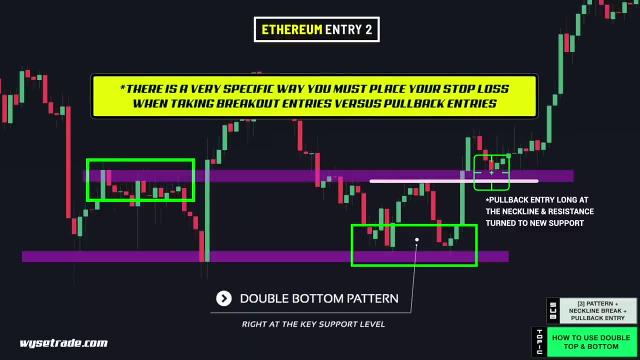 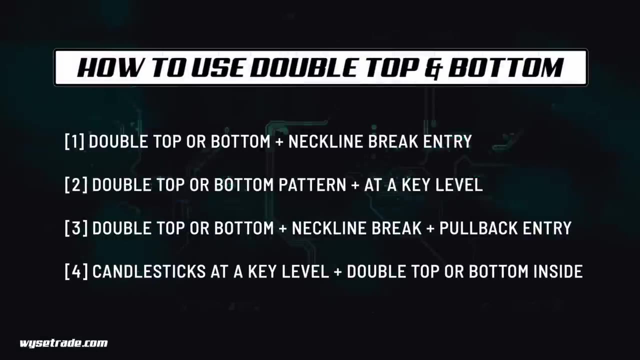 a very good level because it was formed way back here. Now there is a very specific way you must place your stop loss when taking breakout entries, but then a very different way you must place your stop loss when taking pullback entries. So, moving on to the fourth variation, candlestick patterns. 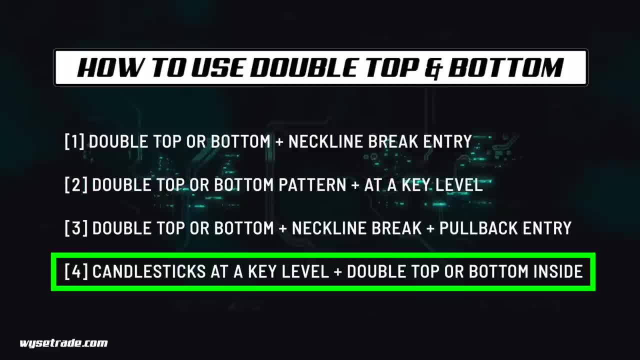 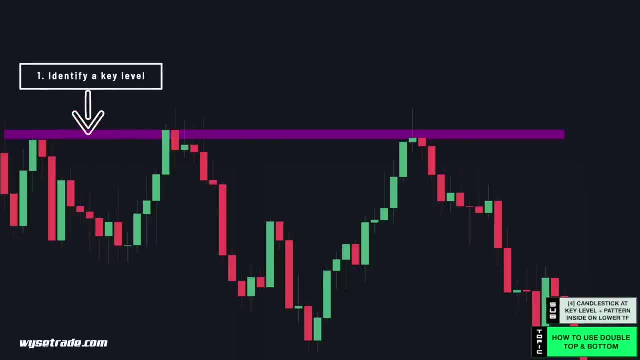 forming at a key level and then a double top or double bottom pattern, but instead of taking the breakout entry, waiting for a pullback entry. So you first look for a key level, which you have through this reversal point here, which gives you a level of resistance As price comes back up to. 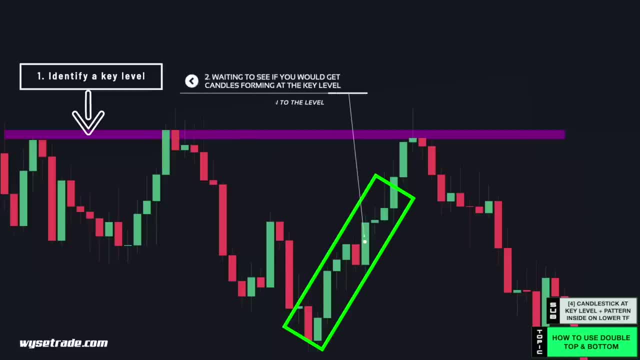 this level. you were waiting to see if you would get candlesticks forming at the level to show a reaction to the level of resistance which you got through this long wick candle. But a reaction does not equal a trade, as price can stall at this key level, form the candle and still break. 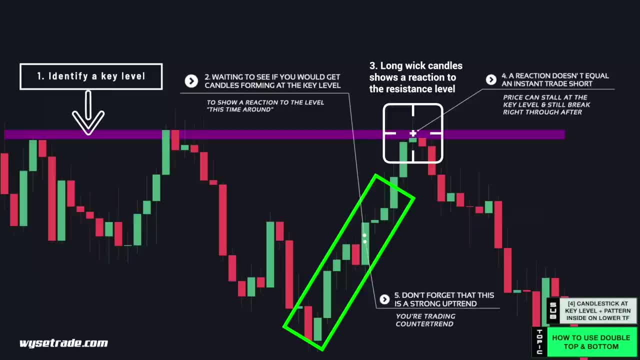 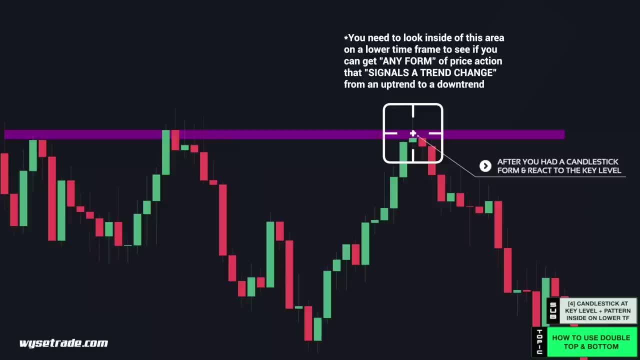 right through. Don't forget that this is a very important level of resistance and it's a very strong uptrend. So what you need to do is, after you have your long wick candle, react to the level of resistance. you need to look inside of this area on the lower timeframes to see if you can. 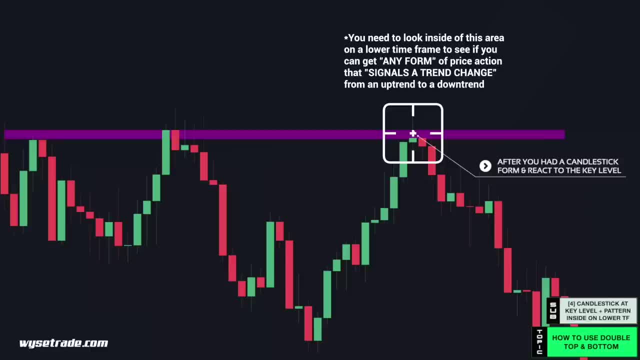 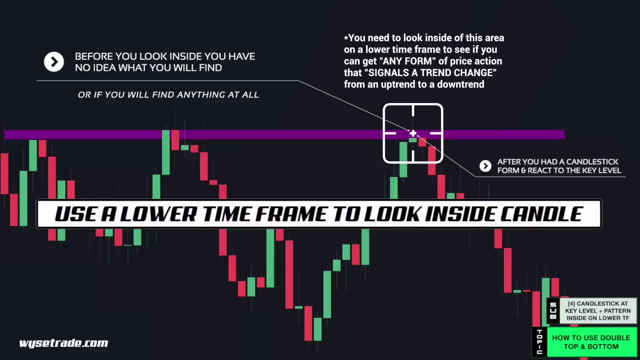 get any form of price action that signals a trend change from an uptrend to a downtrend. Now, this is a very key point: Before you look inside of this area, you have no idea what you will find, or if you will find anything at all. So let's pull up a lower timeframe, specifically the six. 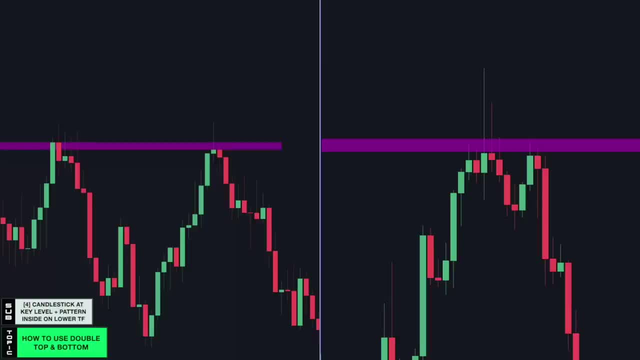 hour timeframe and put it beside this one. So, on the left is the daily timeframe we just looked at And on the right, here is the six hour timeframe of the same asset. This resistance level here is the same resistance level here. This area, here where the candlestick formed, is this same area. 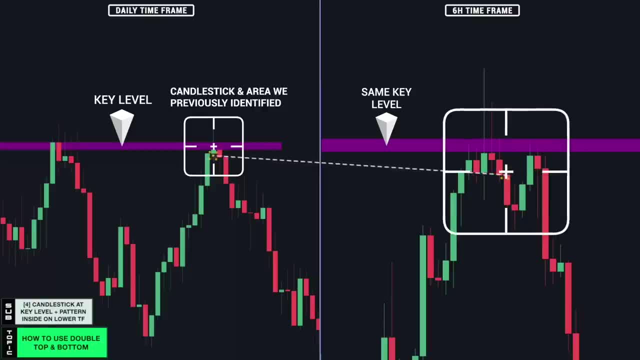 here on the six hour timeframe. Now, the reason we are using a lower timeframe is because on the main timeframe, where we found the initial setup, price movement is too tight, meaning we don't have good swings that give us good price action. that signals a trend change after we had the long wick. 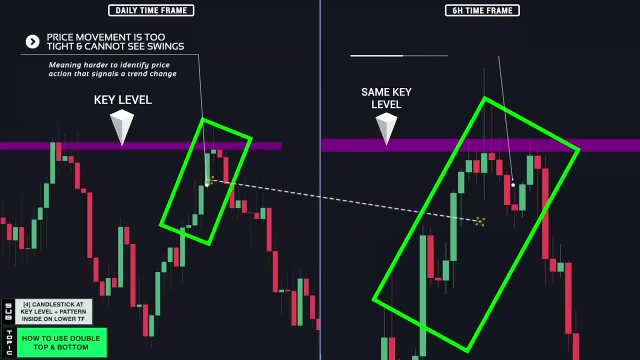 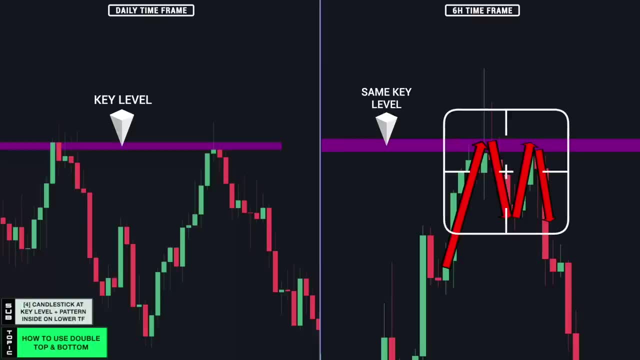 candle, Whereas here, on this lower timeframe on the right, we can see so much more data and see the actual swings of price. So what you had on this lower timeframe was a perfect double top pattern that formed right at the key level of resistance and inside of the long wick candle from. 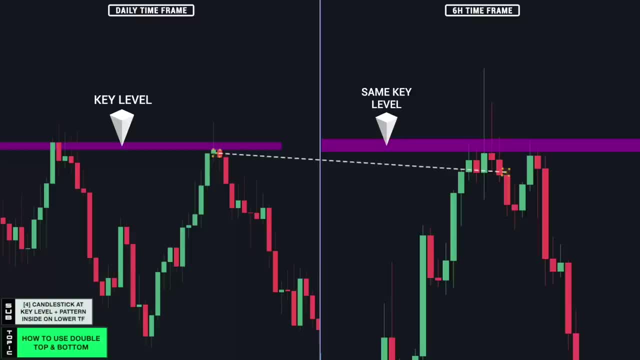 the higher timeframe. So again, to confirm the reversal and the trend change neckline placed here at the swing low. and once price breaks the neckline and makes a lower low, your trend change is confirmed from an uptrend to a downtrend. The breakout here is then when you would go to the lower intraday. 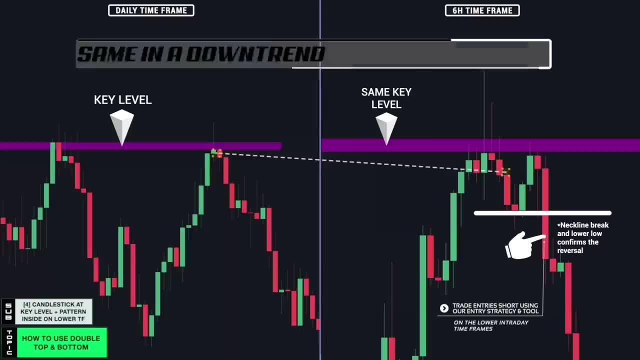 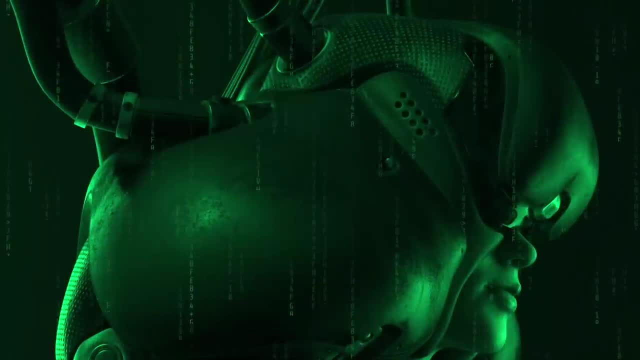 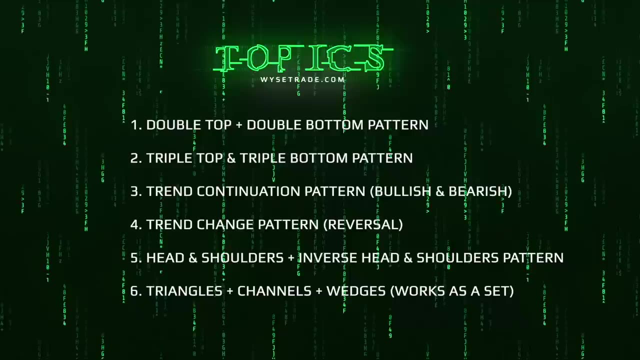 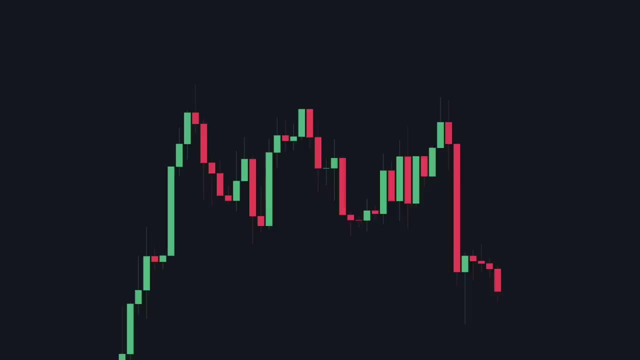 timeframes to take trade entries short. Now going in the opposite direction, in a downtrend, this would work the same. So moving on to the next pattern, the triple top and triple bottom pattern. So before we continue, make sure you go follow our Instagram account at wisetrade to stay notified. 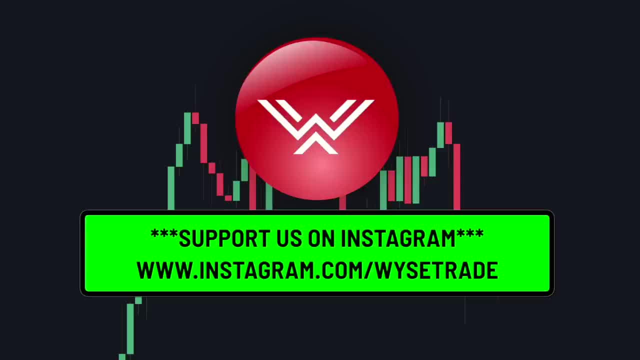 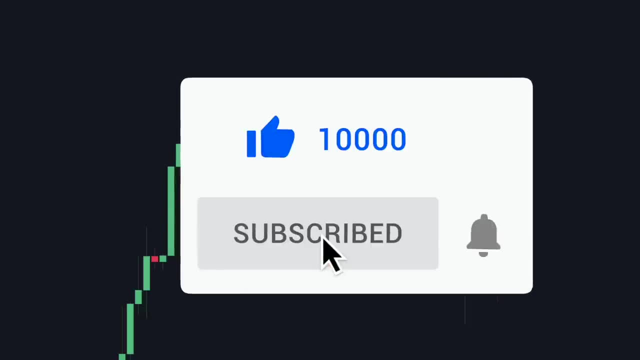 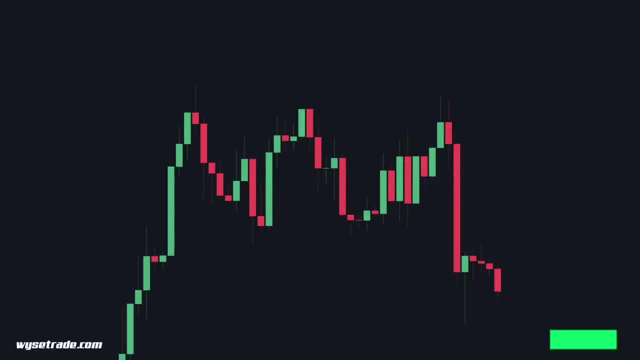 about a lot of big projects we have on the way Now. if you are enjoying this video and want to support our team, hit the like button, subscribe and turn on the notifications bell so that you know exactly when new content is released. Now moving to the next pattern, the triple top and. 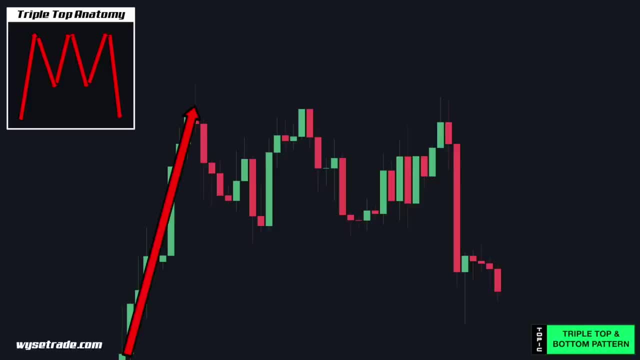 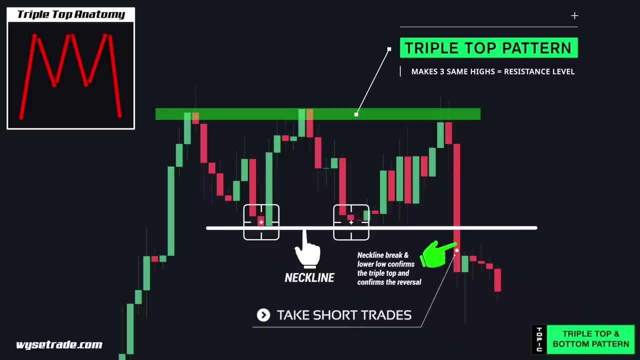 triple bottom pattern. So price is in an uptrend before it makes three same highs in a row, forming the triple top pattern. The swing lows here create the neckline and support level and when it breaks you would take trade entries short, as the reversal is now confirmed. 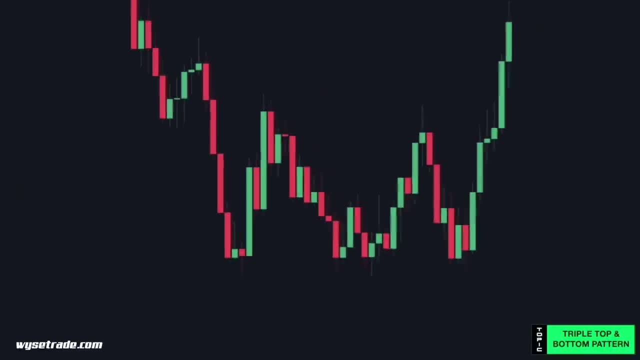 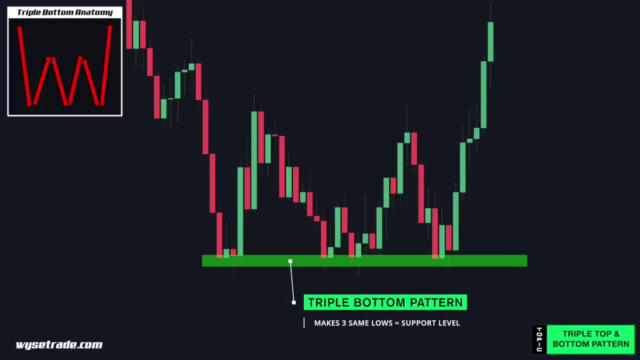 Now going the other way. Price is in a downtrend before it makes three same lows, forming the triple bottom pattern. The swing highs here create the neckline and resistance level and when it breaks you would take trade entries long, as the reversal is now confirmed. 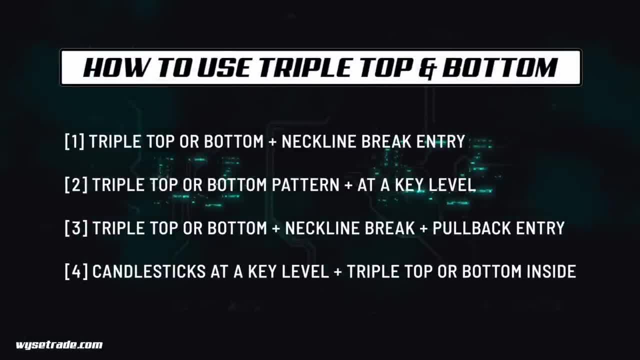 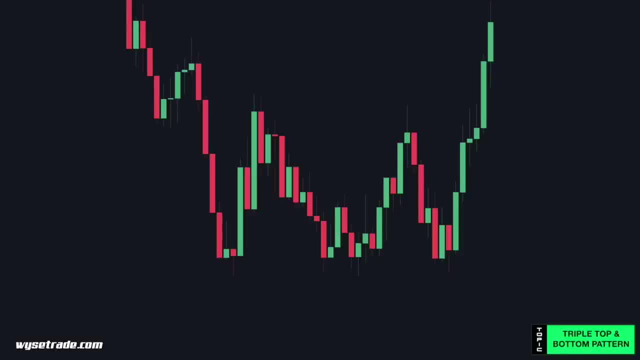 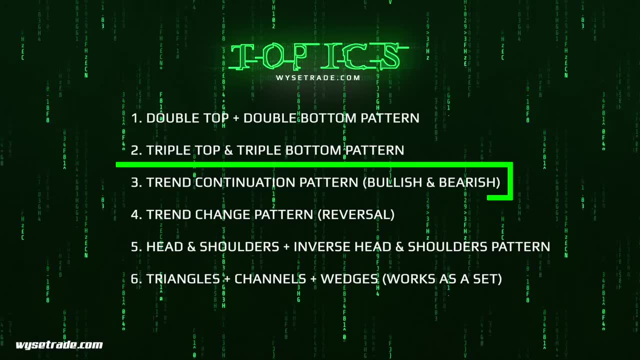 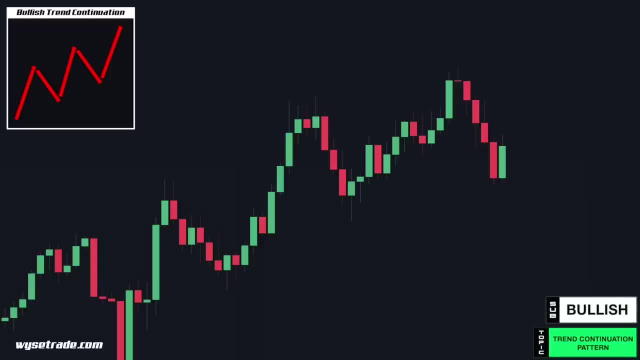 So using the triple top and triple bottom pattern is the same as the four variations we showed you for the double top and double bottom pattern, so we won't go through it again. Moving to the next pattern, the trend continuation pattern. A bullish trend continuation pattern has your runs and pullbacks. 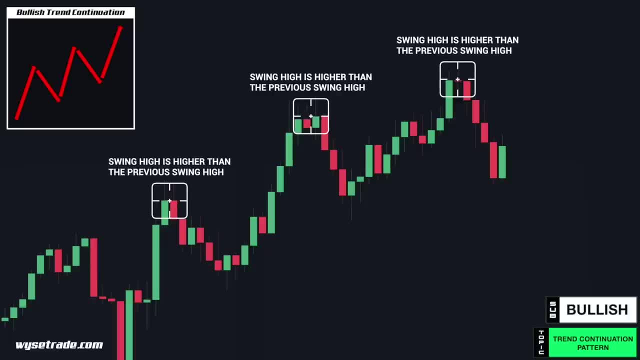 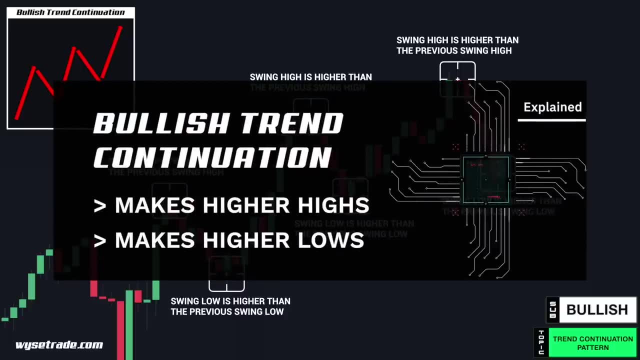 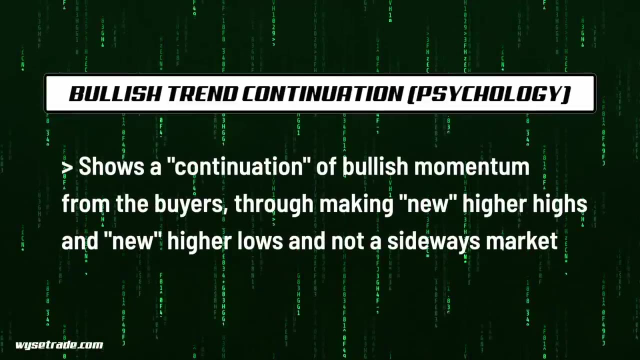 The swing highs are higher than the previous swing highs. The swing lows are higher than the previous swing lows. This means a bullish trend continuation pattern makes higher highs and higher lows. From a price action standpoint it shows a continuation of bullish momentum from the top to. 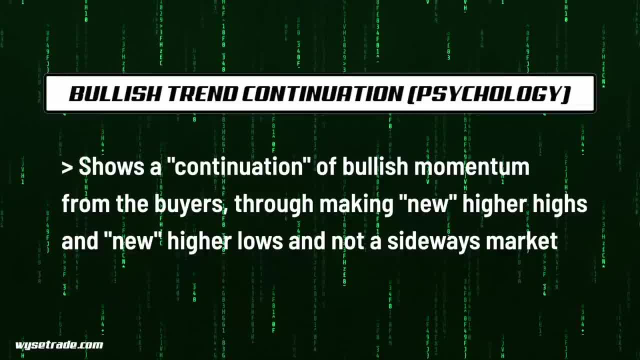 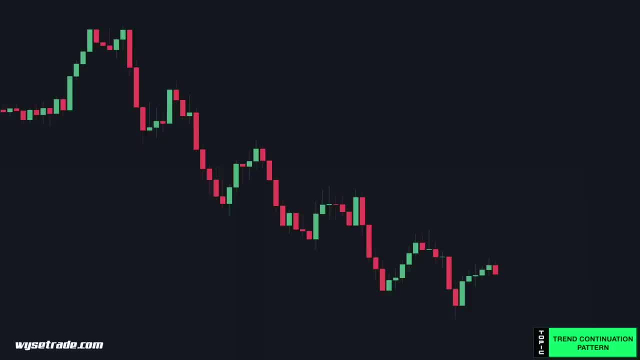 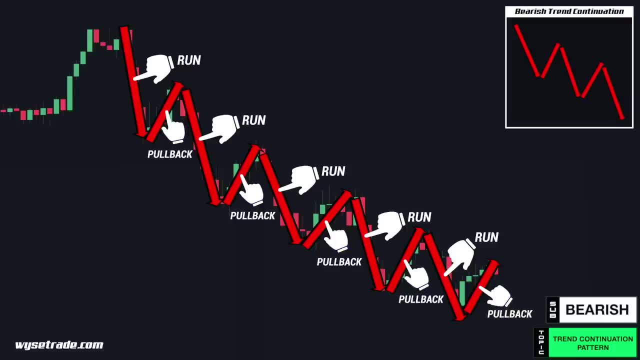 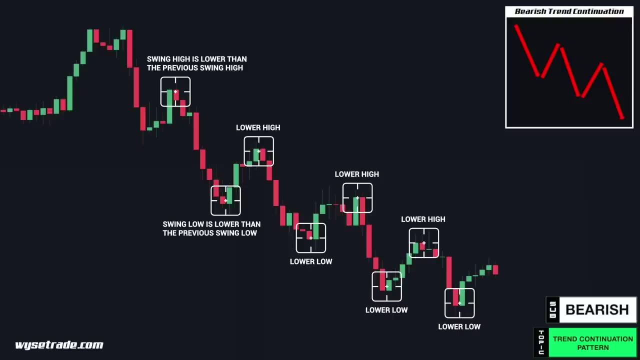 the buyers through making new higher highs and new higher lows and not a sideways market. Now going the other way, A bearish trend continuation pattern has your runs and pullbacks. The swing highs are lower than the previous swing highs. The swing lows are lower than the previous. 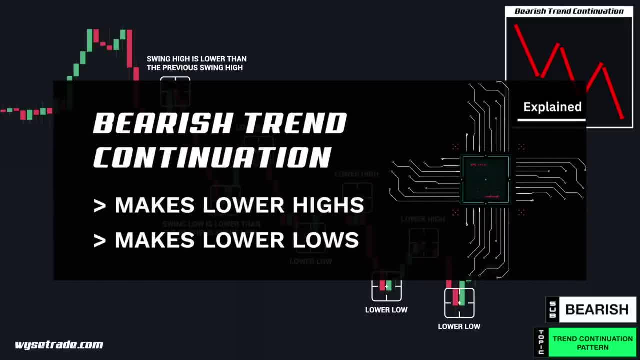 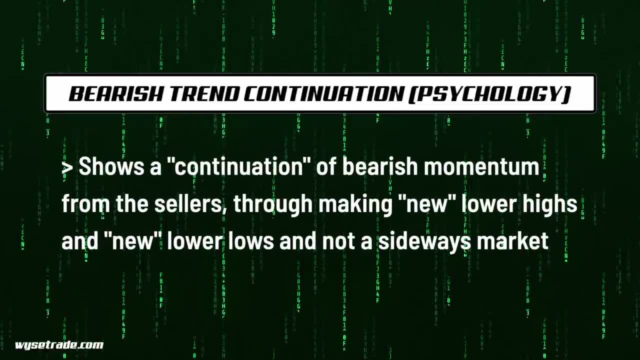 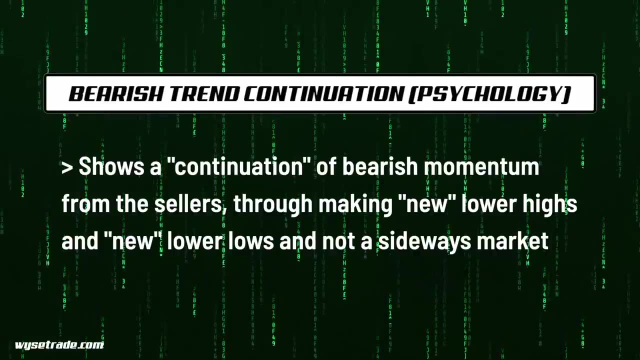 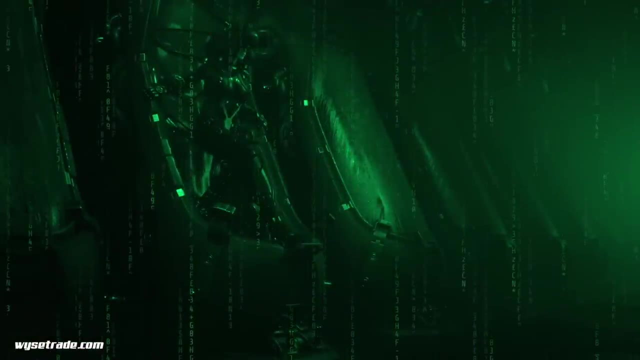 swing lows. This means a bearish trend continuation pattern Makes lower highs and lower lows. So from a price action standpoint it shows a continuation of bearish momentum from the sellers through making new lower highs and new lower lows and not a sideways market. Now moving to the next pattern, the trend change pattern. 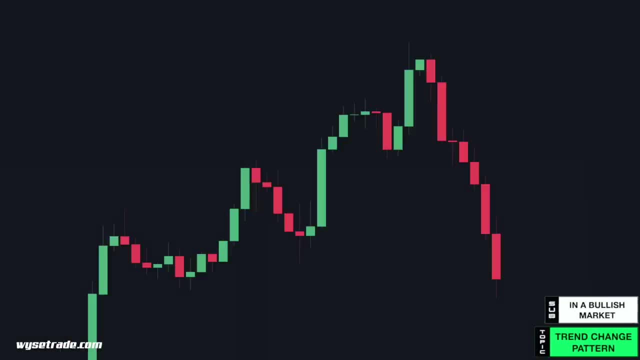 In a bullish market there are two ways the trend change pattern can form. Variation one: You have your moving uptrend through the higher highs and higher lows before price makes a lower low, giving you your trend change pattern in a bullish market. 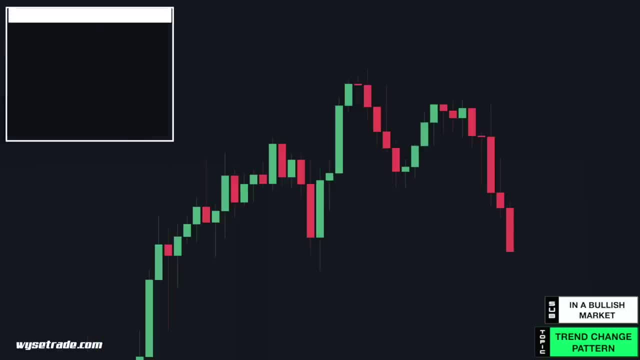 Now variation two. You again have your moving uptrend through higher highs and higher lows before price makes both a lower high and higher lows and a lower low, giving you your trend change pattern in a bullish market. So from a price action standpoint it shows a loss of momentum from the buyers as price. 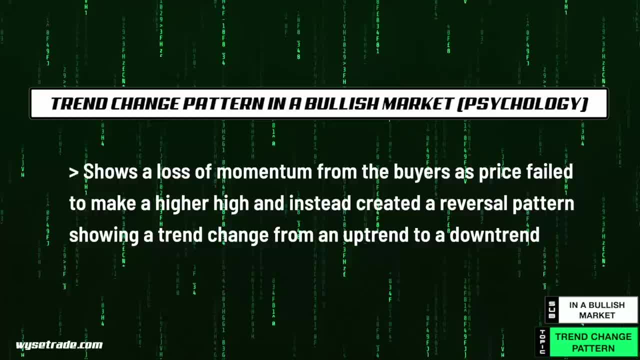 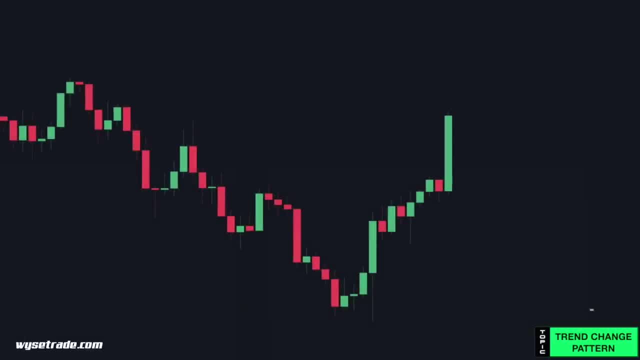 failed to make a new higher high and instead created a reversal pattern, Now going the other way. In a bearish market, there are two ways the trend change pattern can form Variation. 1. You have your moving downtrend through lower highs and lower lows. 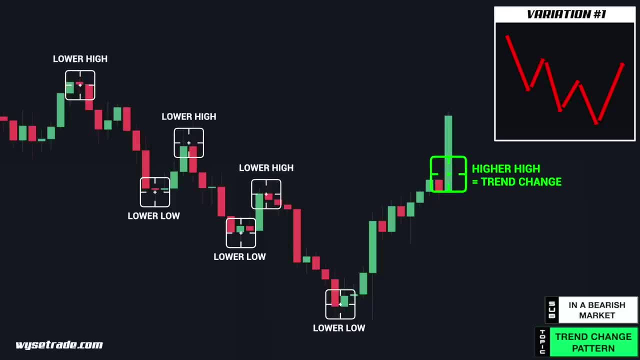 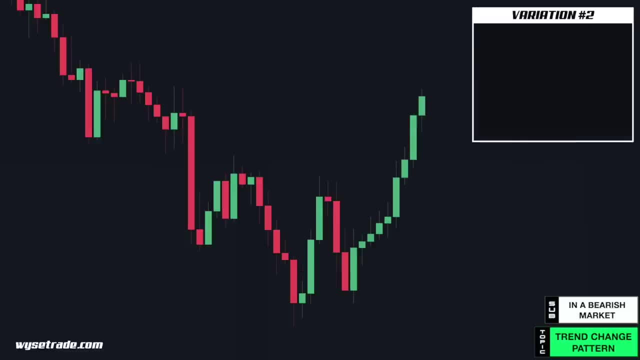 before price makes a higher high, giving you your trend change pattern in a bearish market. Now variation 2.. So you have your moving downtrend again through lower highs and lower lows, before price makes both a higher low and a higher high, giving you your trend change pattern in a 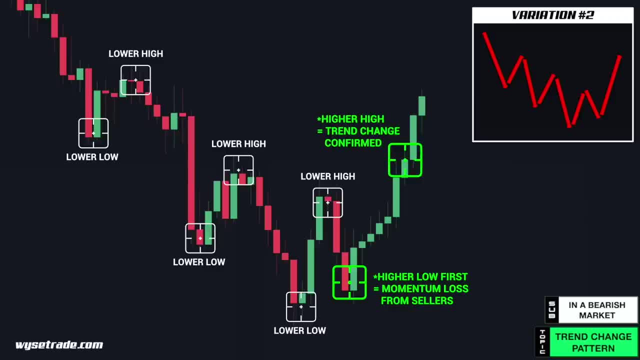 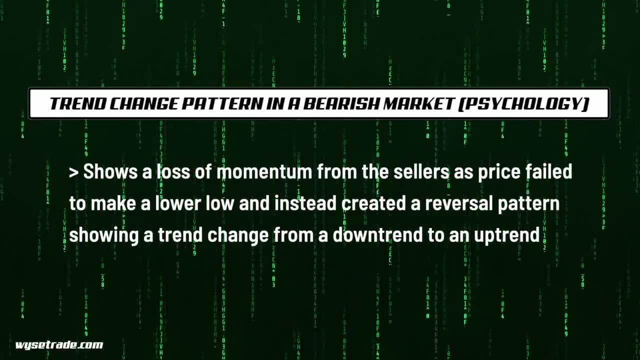 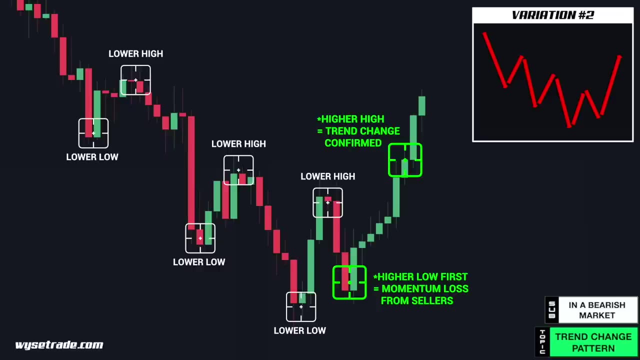 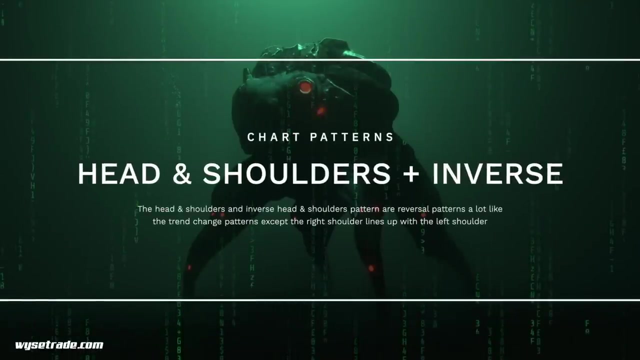 a bearish market. so from a price action standpoint it shows a loss of momentum from the sellers as price failed to make a lower low and instead created a reversal pattern showing a trend change from a downtrend to an uptrend. so moving on the head and shoulders and inverse head and shoulders. 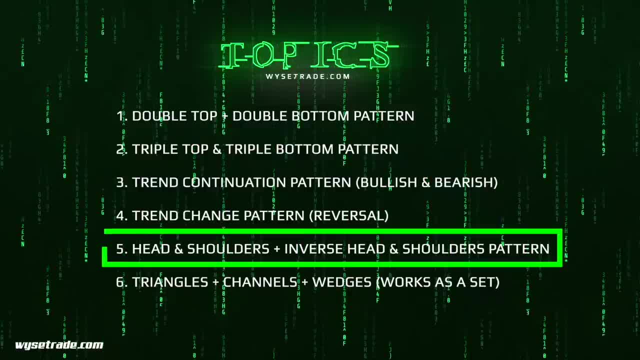 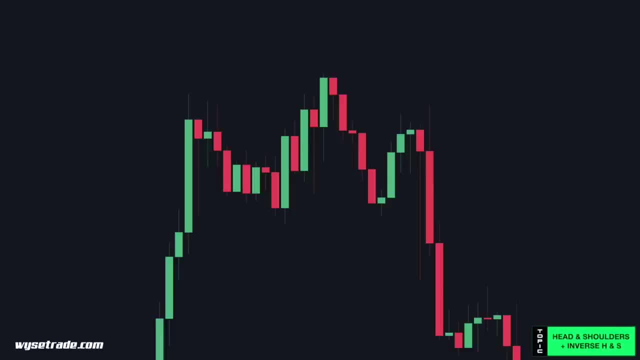 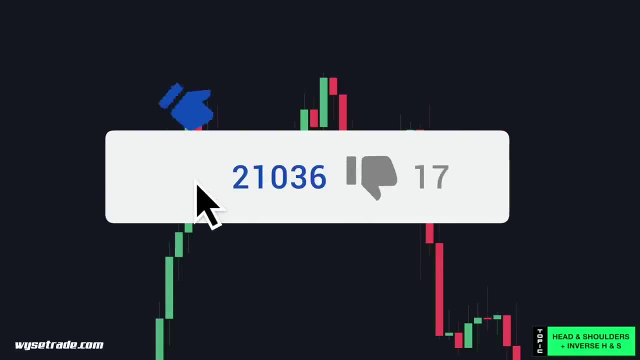 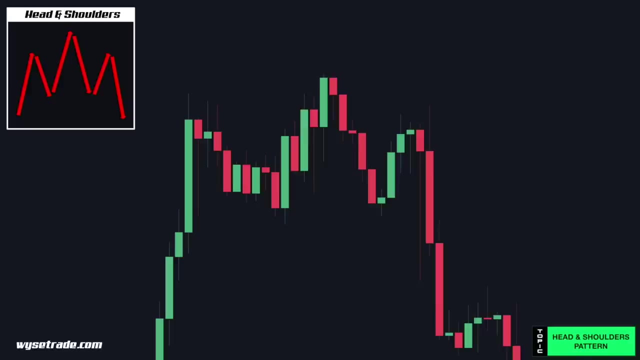 pattern. so before we continue, if you are enjoying this video and want to show your support, please hit the like button right now. so the head and shoulders pattern starts with your moving uptrend: left shoulder, the head at the swing high and then the right shoulder at the lower high. the swing lows here make a neckline or support level. 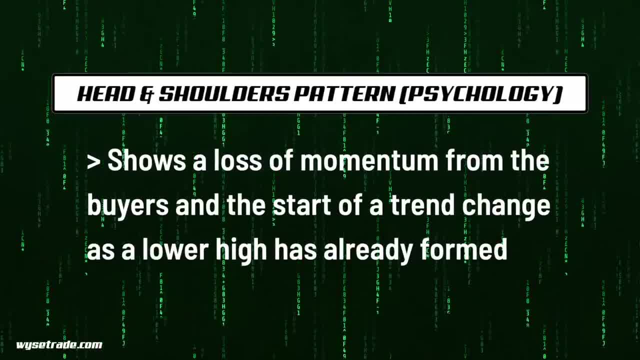 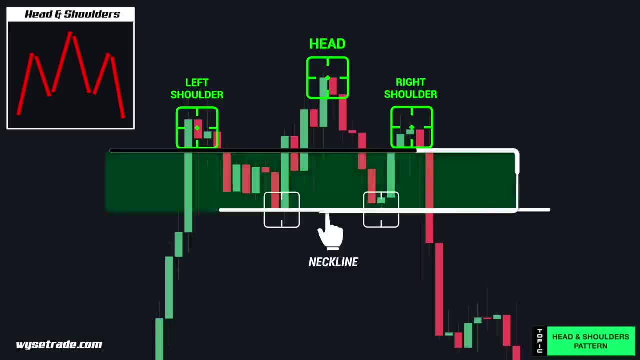 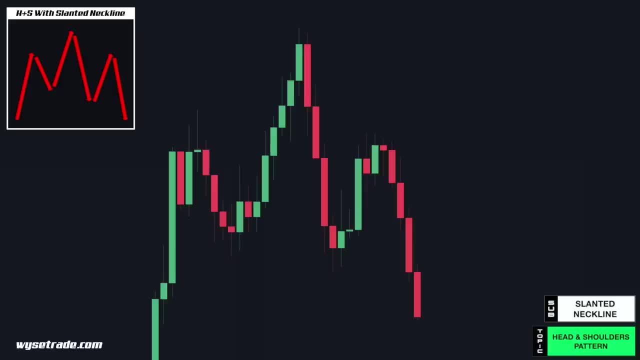 from a price action standpoint, it shows a loss of momentum from the buyers and the start of a trend change, as a lower high has already formed. now there is a higher quality head and shoulders pattern, which is a head and shoulders pattern with a slanted neckline. it's the same as the normal head and shoulders pattern, except you already have. 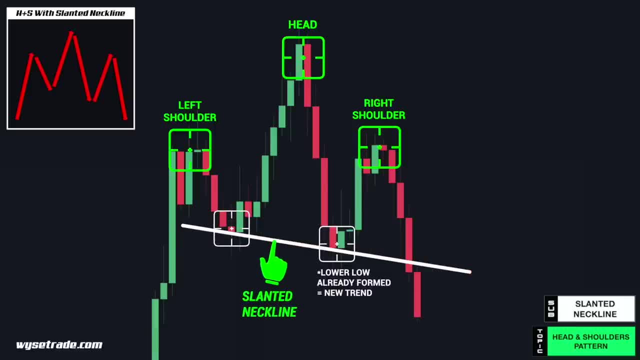 a lower low and then the right shoulder at the lower high. the swing lows here make a neckline, and then the left shoulder at the lower high. the swing lows here make a head and shoulders pattern that formed, creating the slanted neckline. from a price action standpoint, this is a higher quality. 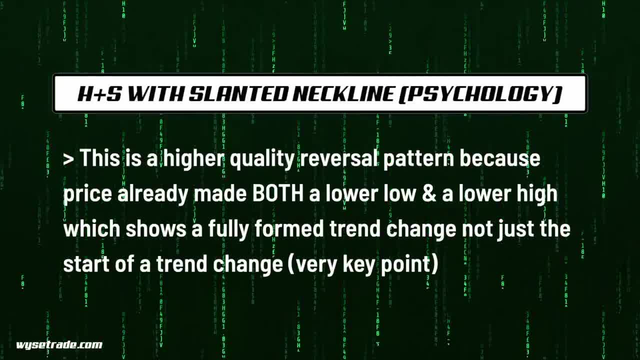 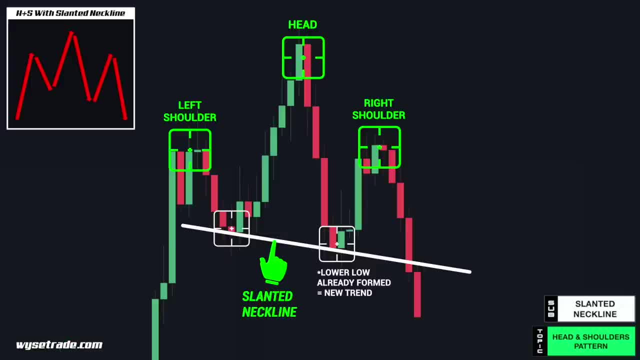 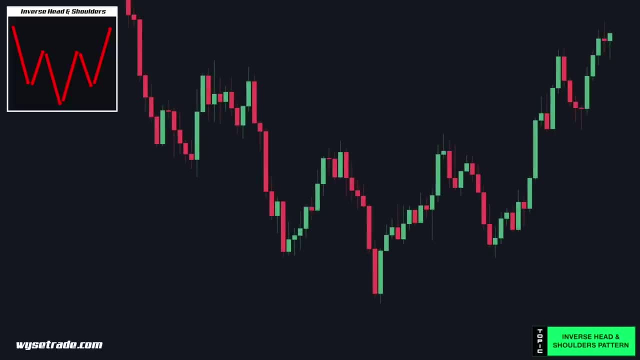 reversal pattern because price already made both a lower low and lower high, which shows a fully formed trend change, not just the start of a trend change now going in the opposite direction, the inverse head and shoulders pattern starts with your moving downtrend left shoulder, the head at the. 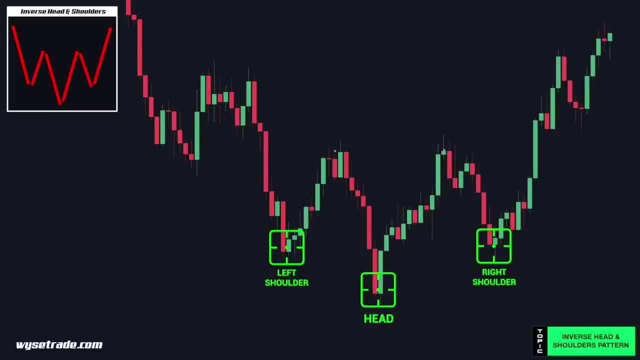 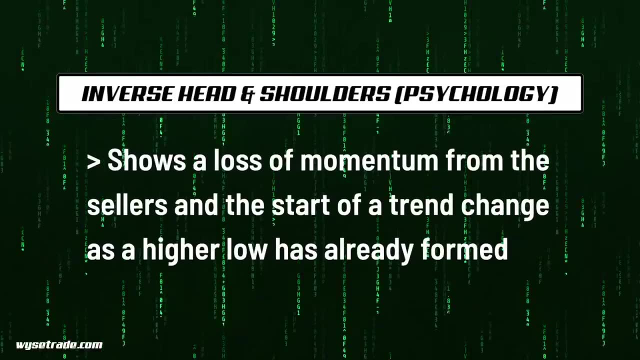 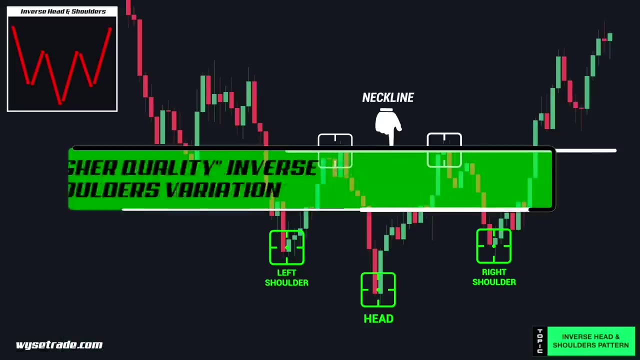 swing low and then the right shoulder at the higher low. The swing highs make a neckline or resistance level. So from a price action standpoint it shows a loss of momentum from the sellers and the start of a trend change as a higher low has already formed. Now again there is a higher 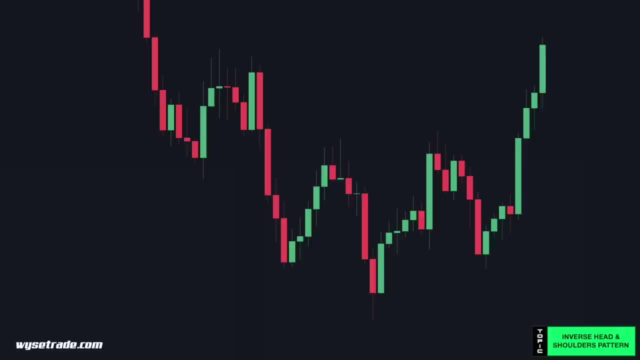 quality inverse head and shoulders pattern, which is an inverse head and shoulders pattern with a slanted neckline. Again, it is the same as your normal inverse head and shoulders pattern, except you already have a higher high that formed creating the slanted neckline. Now from a price. 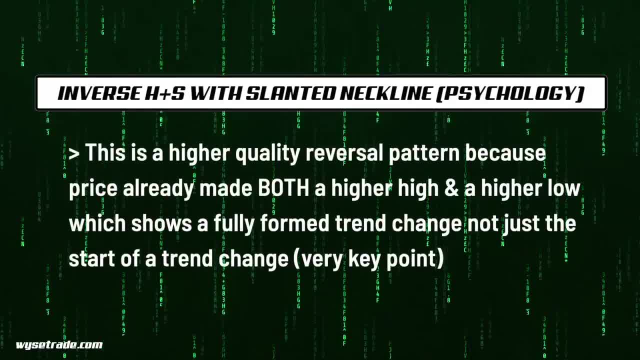 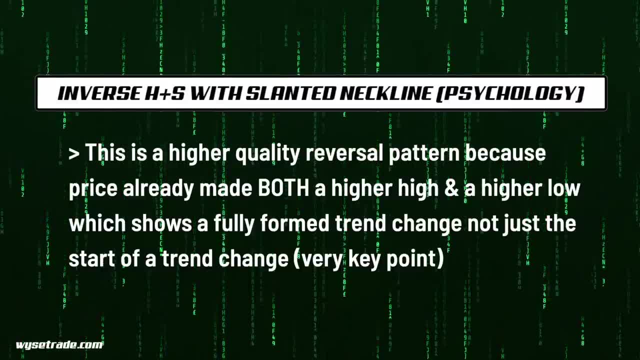 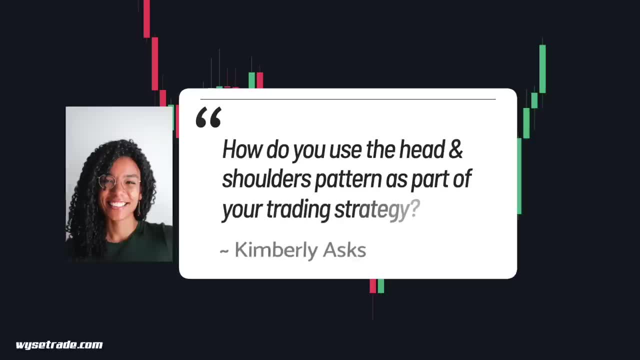 action standpoint, this is a higher quality reversal pattern, because price already made both a higher high and higher low, which shows a fully formed trend change, not just the start of a trend change. So this then brings us to our next question, which is: how do we use the head and 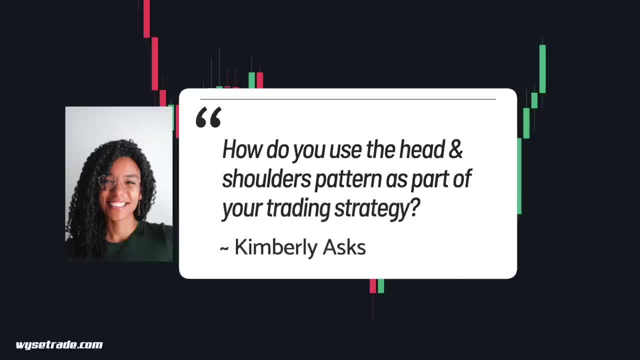 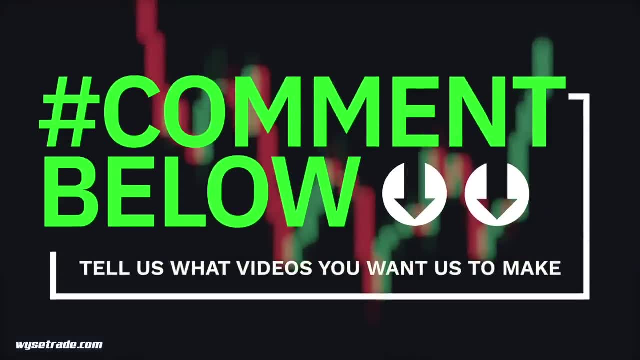 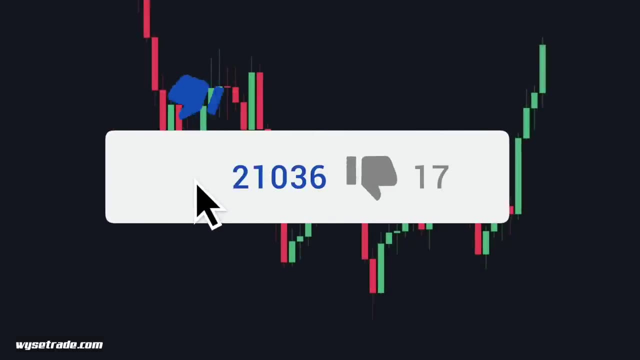 shoulders pattern as part of our strategy. Again, right now, go to the comments below and let us know what you think. If you have any questions, feel free to post them in the comments section below. Also, if you are enjoying this video, hit the thumbs up button to show your support. 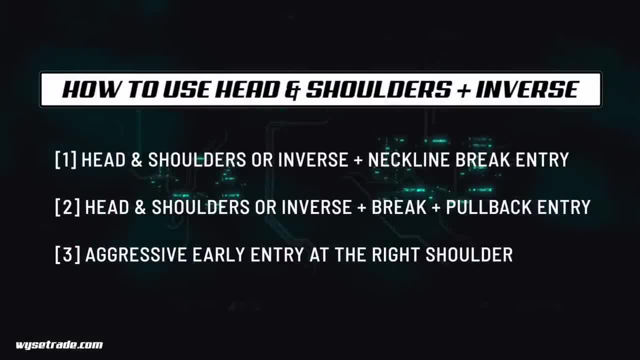 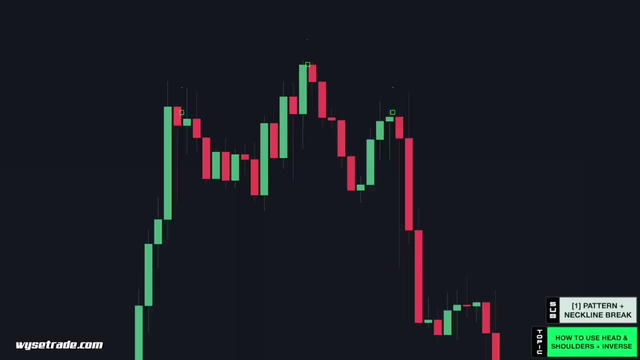 Now these are the three core variations to using the head and shoulders pattern. Let's start with the first, which is the neckline break entry. You first have your head and shoulders pattern that forms Neckline here because of the two points, And once price breaks the neckline and makes a lower low, you would take a breakout. 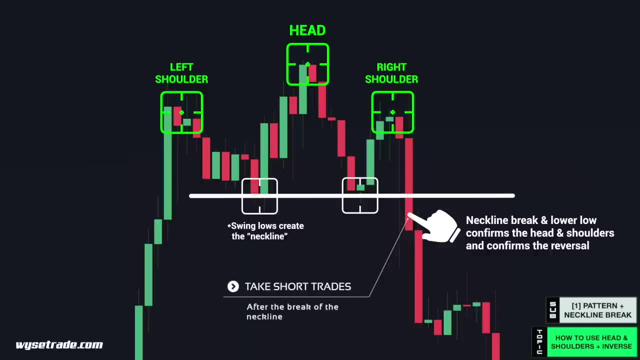 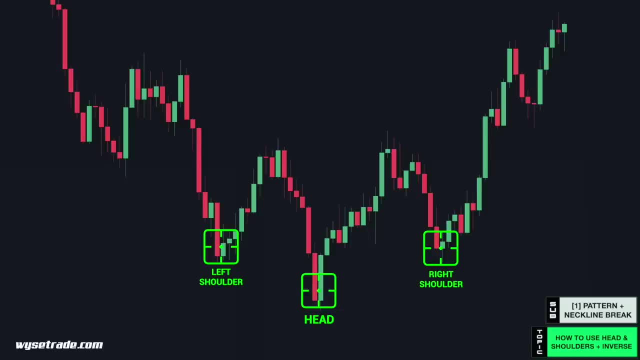 entry short, as the reversal and trend change is now confirmed. Going the other way, You first have your inverse head and shoulders pattern that forms Neckline here because of these two points, And once price breaks the neckline and makes a higher high, you would take a breakout entry long, as the reversal and trend change is now confirmed. 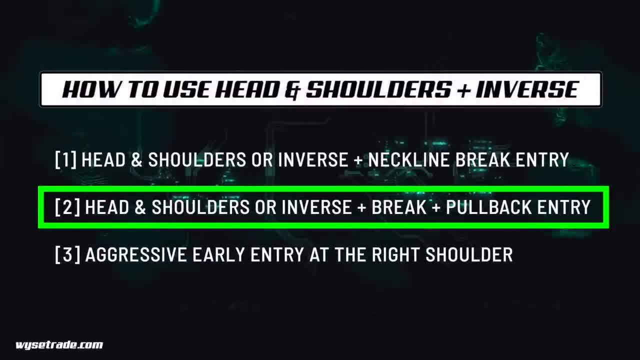 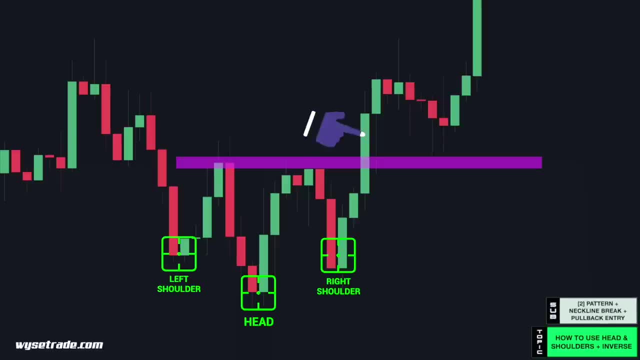 So, moving to the second variation, A head and shoulders or inverse head and shoulders pattern, followed by a neckline break, but instead of taking the breakout entry, waiting for a pullback entry. So you first have your inverse head and shoulders pattern, Neckline here, neckline break, But instead of taking the breakout entry, 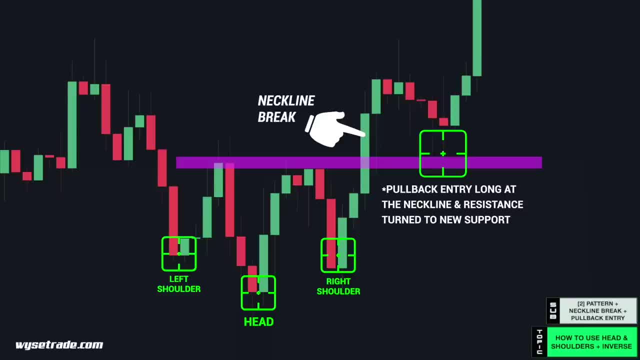 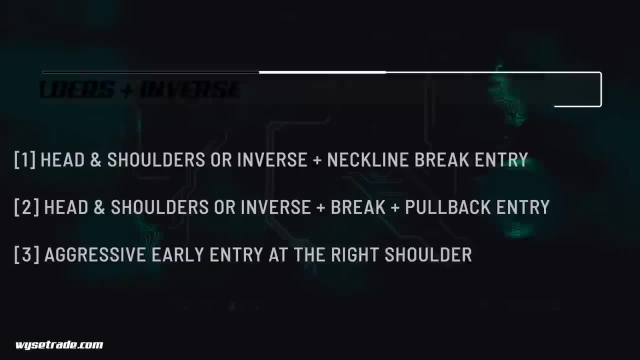 there was a second long entry on the pullback to the new support level, Now going in the opposite direction. this would work the same. So moving on to the third variation, Which is an aggressive early entry at the right shoulder of the pattern, 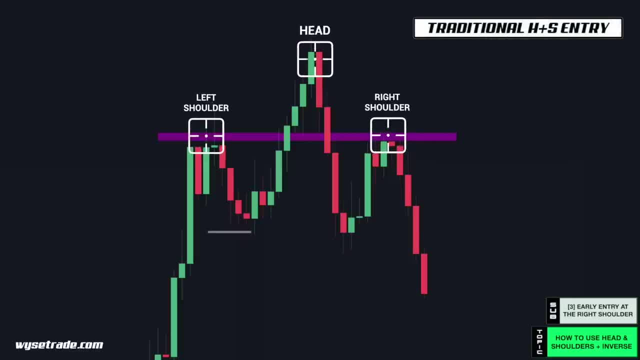 So your regular entry would be identifying the head and shoulders pattern and taking a trade entry short at the break of the neckline here. But now there is a more advanced way to trade the head and shoulders, which is what we call an early aggressive entry right at the right shoulder of 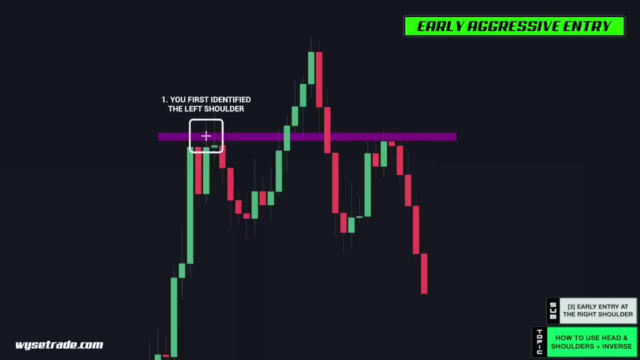 the pattern here, So let's break it down. You first identify the left shoulder and then the head. Now. Now, here's the key. the left shoulder here already makes a resistance level, so you would have had it drawn in and extended out. 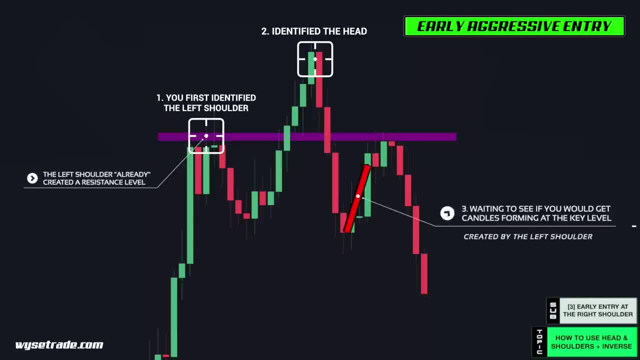 As price comes back up to this resistance level. you would wait to see if you would get candlesticks forming at the level created by the left shoulder, which you got through the multiple long wick candles forming at the level. Then at this point you would look inside of this area to look and see if you get any form. 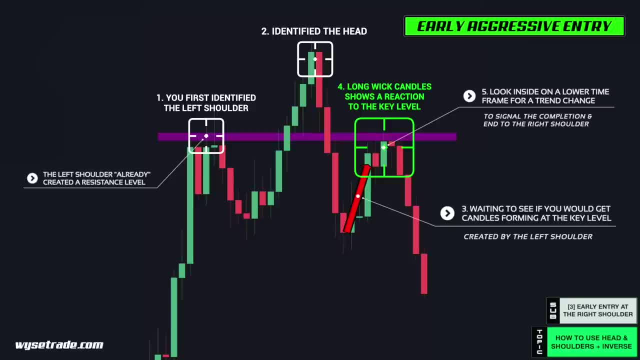 of price action. that signals a trend change to confirm that this right shoulder has completed. So let's pull up a lower time frame, specifically the 4 hour time frame, and put it beside this one. On the left is the daily time frame we just looked at and on the right is the 4 hour. 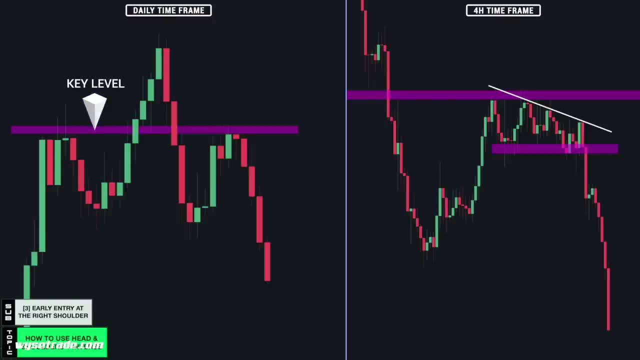 time frame of the same asset. This resistance level here is this same resistance level here. This area here where the candlesticks formed, is this same area here on the 4 hour time frame. Now, On the 4 hour time frame, you had a perfect descending triangle pattern that formed right. 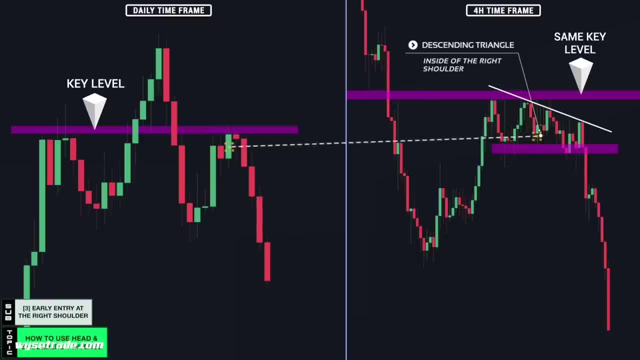 at the right shoulder and resistance level from the higher time frame. When the pattern breaks below, this reversal from an uptrend to a downtrend is now confirmed and also confirms the completion of the right shoulder from the higher time frame. Now, after you had the break, you would go to the lower intraday time frames to take. 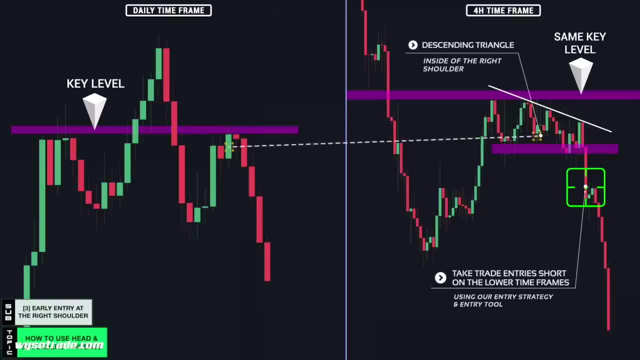 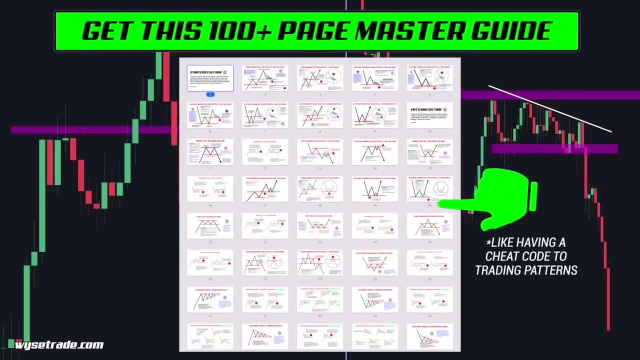 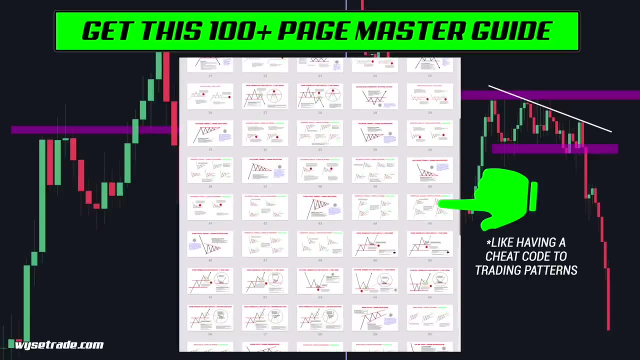 trade entries short using our entry strategy and tool. So, before we continue, Don't forget that there is an over 100 page patterns trading guide that works in combination with this video and goes through every small detail, including exactly where to enter and exit. 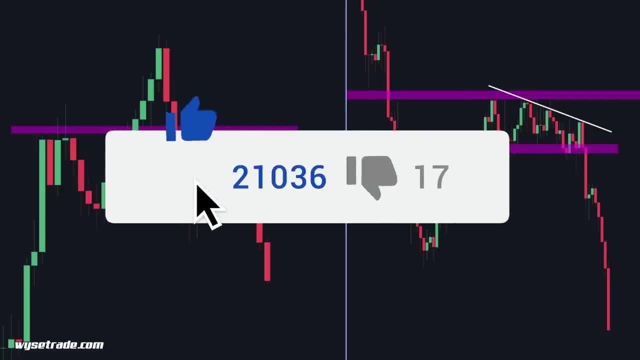 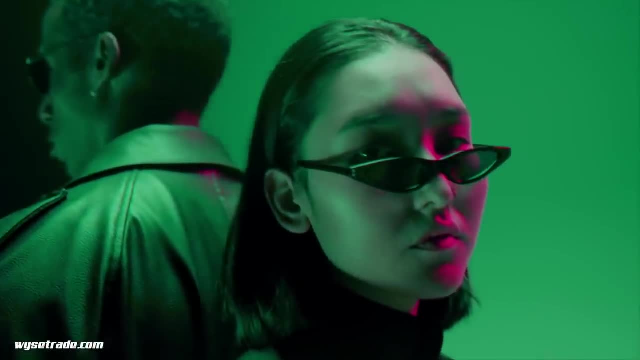 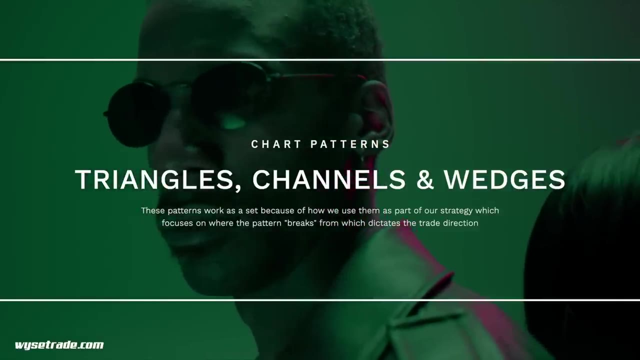 Again, if you're enjoying this video, make sure to hit the thumbs up button to show your support. Now, moving on to the next section: Triangles, Channels and Wedges. These patterns work as a set because of how we use them as part of our strategy. 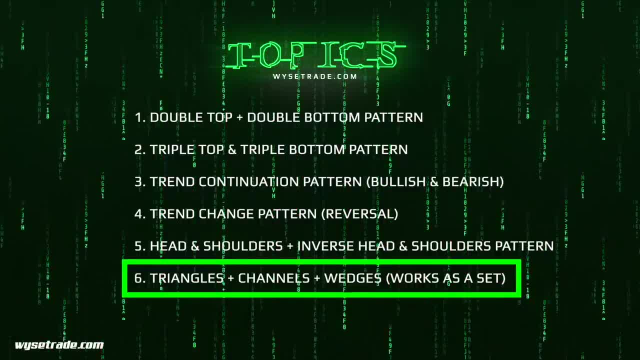 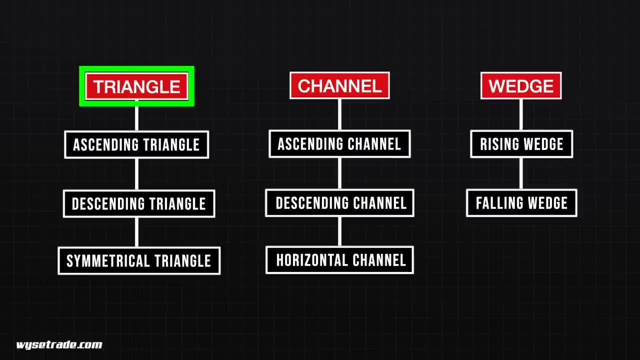 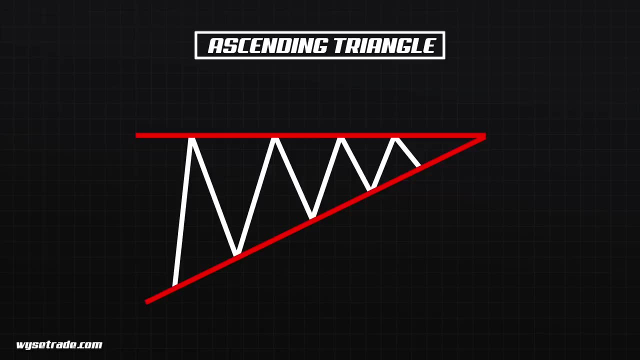 And you'll see why. So let's first go through the three core patterns, starting with the triangle pattern. Now, the triangle pattern has its three variations as well. So we'll start with the ascending triangle. So the top side of the ascending triangle makes same highs and creates a horizontal. 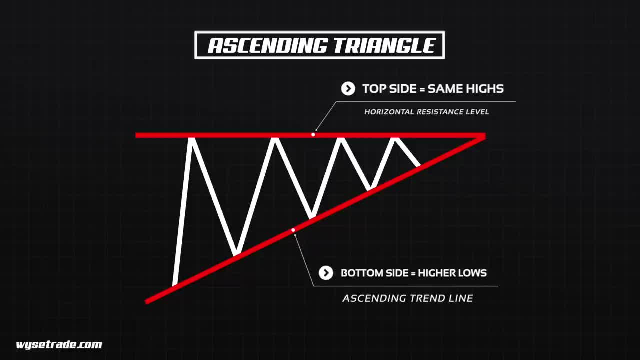 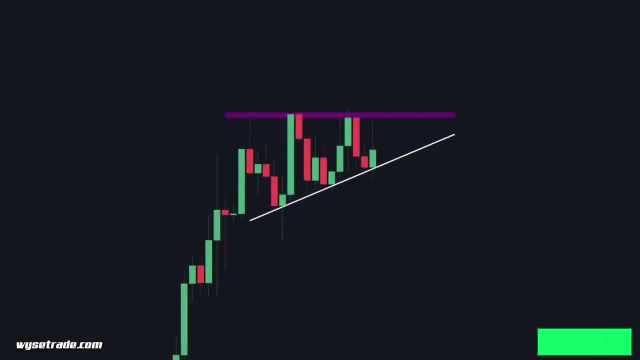 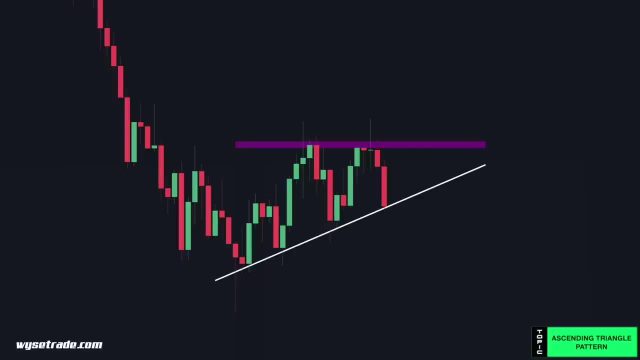 resistance level. The bottom side of the pattern makes higher lows and allows for an ascending trend line to be placed. This pattern then forms in both bullish and bearish markets. The bullish ascending triangle starts with an uptrend, followed by the pattern formation. 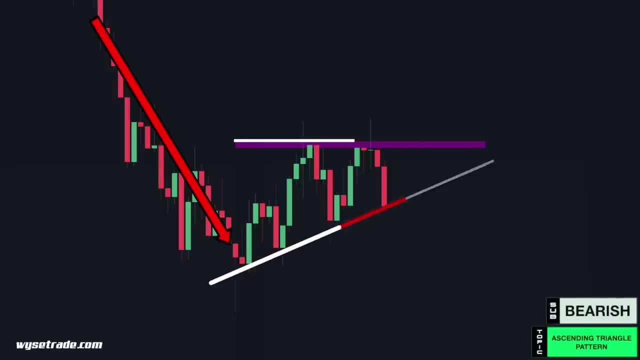 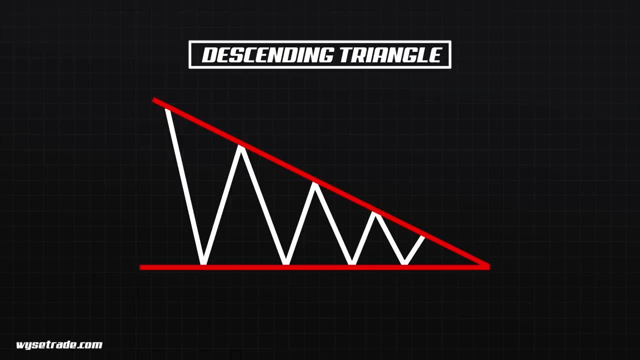 The bearish ascending triangle starts with a downtrend, followed by the pattern formation. So next the descending triangle pattern. The bottom side of the descending triangle makes same lows and creates a horizontal support level. The top side of the pattern makes lower highs and allows for a descending trend line to be placed. 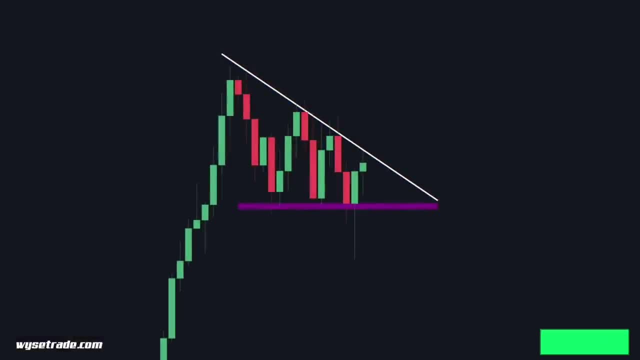 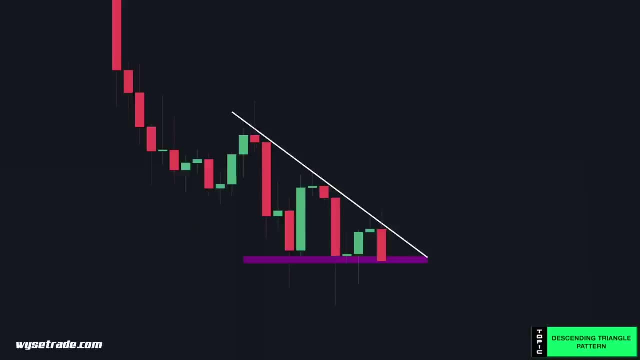 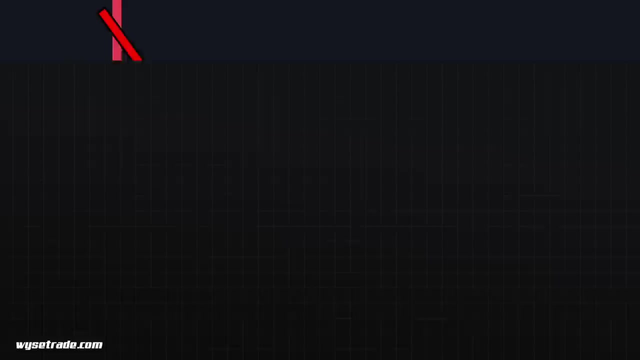 This pattern then forms in both bullish and bearish markets. A bullish descending triangle starts with an uptrend, followed by the pattern formation. A bearish descending triangle starts with a downtrend, followed by the pattern formation. So next the symmetrical triangle pattern. 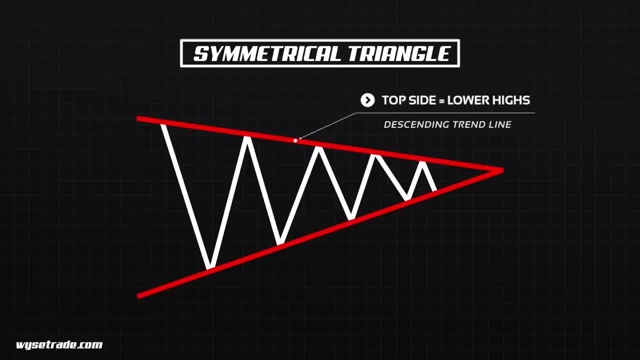 The top side of the symmetrical triangle makes lower highs, Which allows for a descending trend line to be placed above. The bottom side of the pattern makes higher lows, which allows for an ascending trend line to be placed below. This pattern then forms in both bullish and bearish markets. 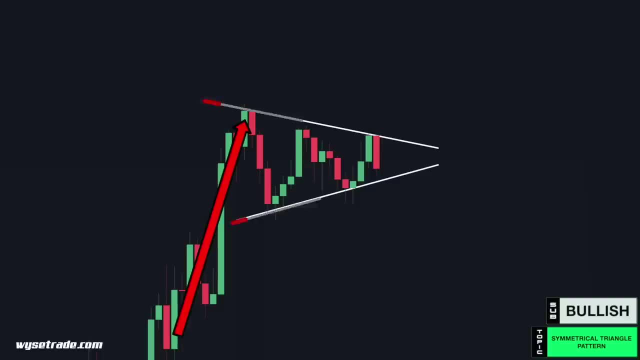 A bullish symmetrical triangle starts with an uptrend, followed by the pattern formation. The bearish symmetrical triangle starts with a downtrend, followed by the pattern formation. So we'll be showing you how to use these all once we get to the strategies section. 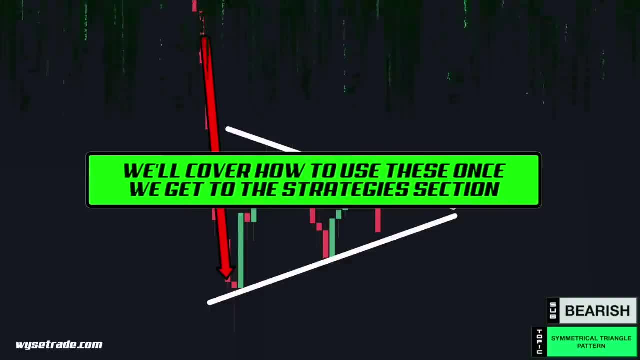 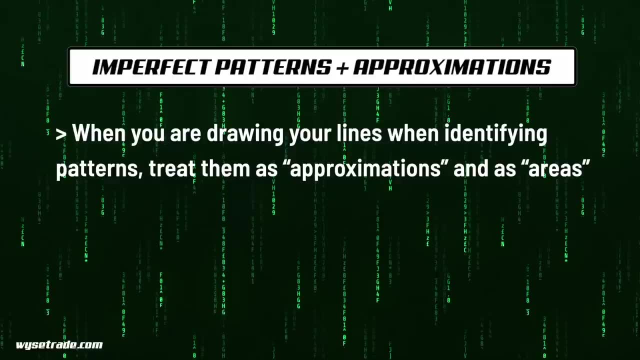 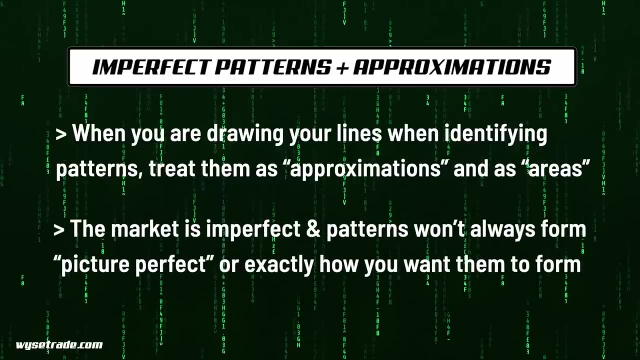 Now, let's get started Now, before we continue. this is the most important concept of this entire video. When you are drawing your lines, when identifying patterns, treat them as approximations and as areas. The reason for this is because the market is imperfect and patterns won't always. 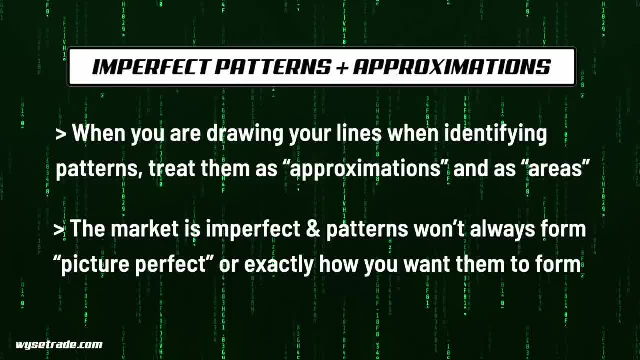 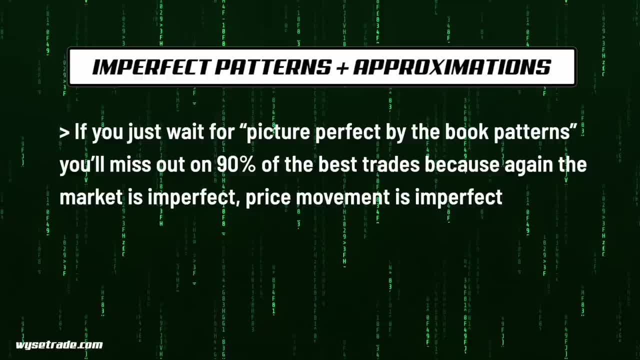 form, picture perfect or exactly how you want them to form. If you just wait for picture perfect by the book patterns, you'll miss out on 90% of the best trades Because, again, the market is imperfect. So let's get started. 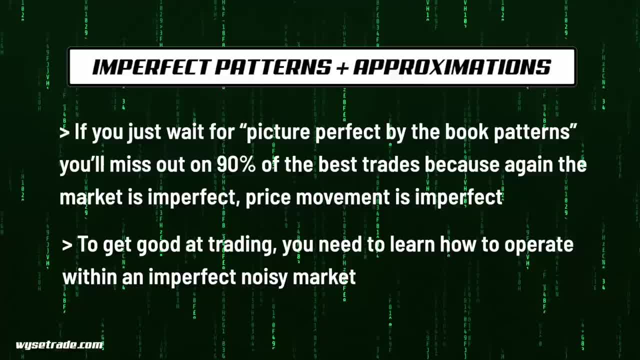 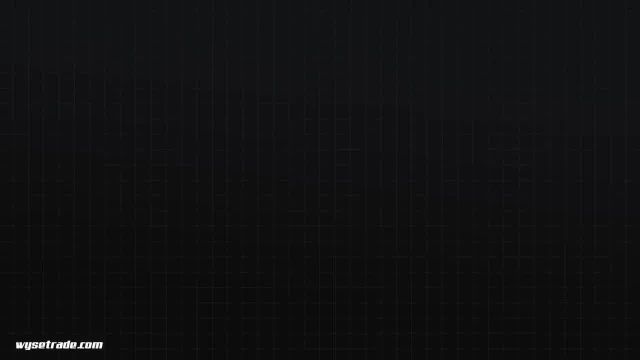 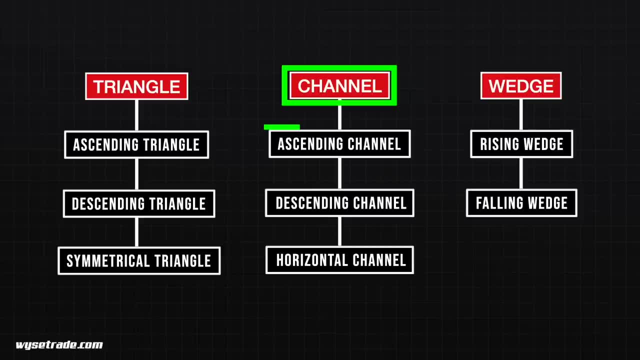 The market is imperfect and to get good at trading, you need to learn how to operate within an imperfect, noisy market. Moving on to the next pattern, which is the channel pattern. Now, the channel pattern has three variations. Let's start with the first, which is the ascending channel pattern. 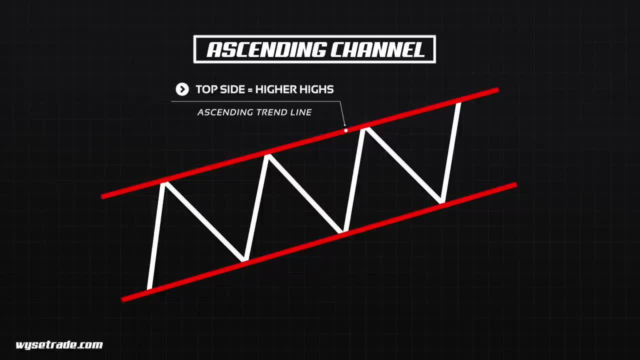 So the top side of the ascending channel makes higher highs, which allows for an ascending trend line to be placed. The bottom side of the pattern makes higher lows, which also allows for an ascending trend line to be placed. The two trend lines are parallel to each other and are both in an upwards direction. 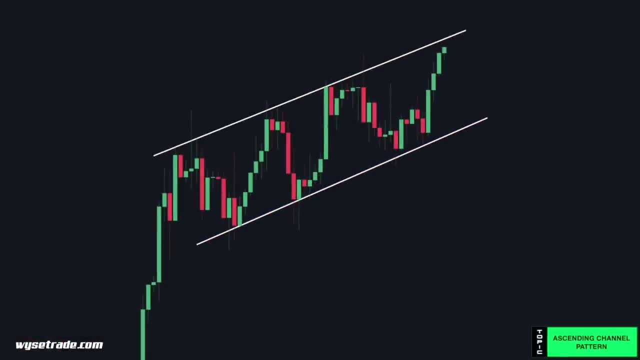 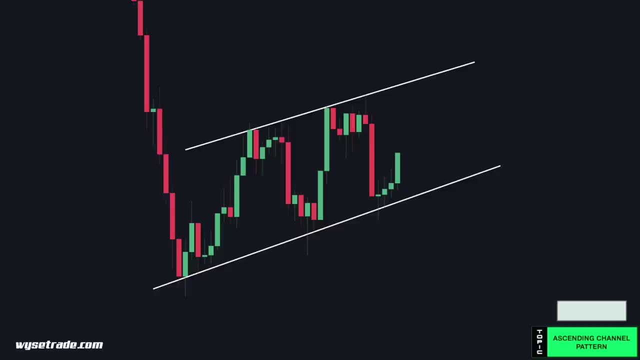 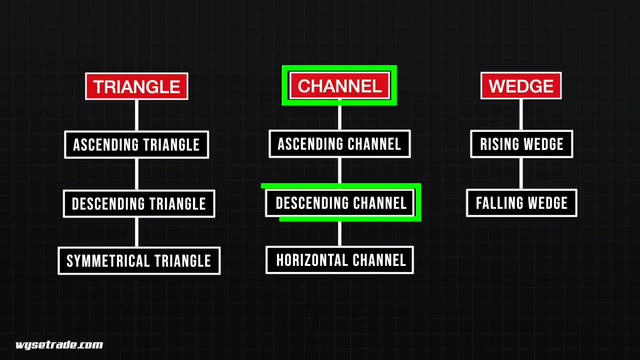 This pattern then forms in both bullish and bearish markets. A bullish ascending channel starts with an uptrend, followed by the pattern formation. A bearish ascending channel starts with a downtrend, followed by the pattern formation. So next the descending channel pattern. 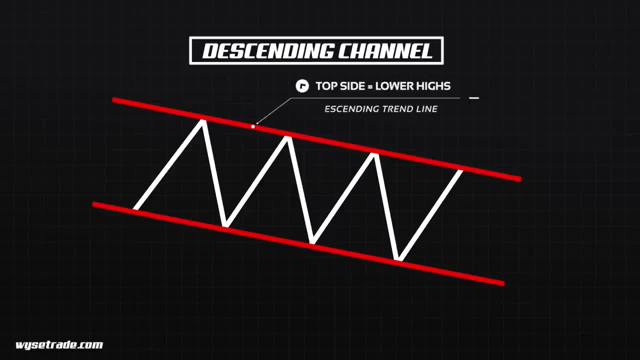 The top side of the descending channel makes lower highs, which allows for a descending trend line to be placed. The bottom side of the pattern makes lower lows, which allows for a descending trend line to be placed. The two trend lines are parallel to each other and are both in a downwards direction. 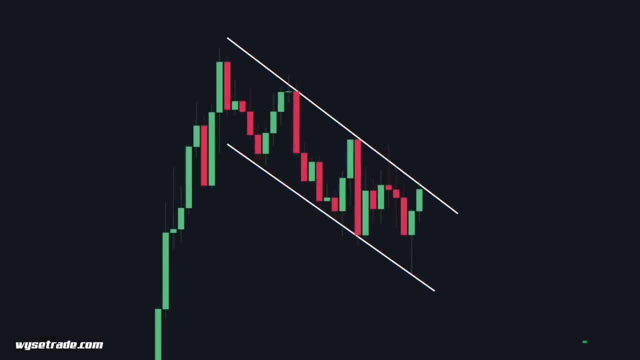 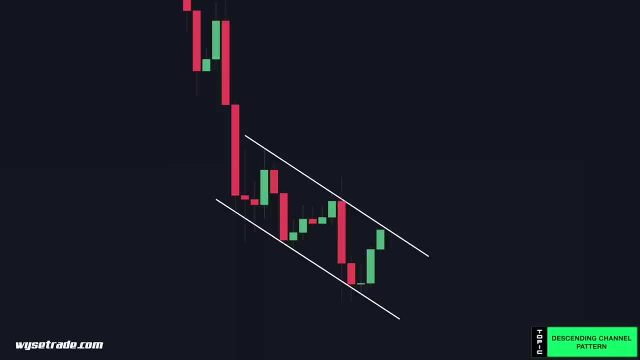 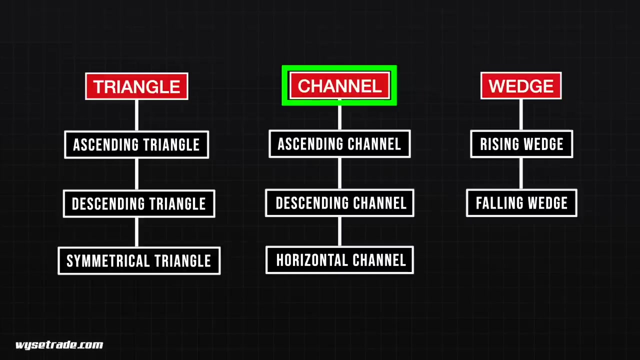 This pattern then forms in both bullish and bearish markets. A bullish descending channel starts with an uptrend, followed by the pattern formation. A bearish descending channel starts with a downtrend, followed by the pattern formation. So next the horizontal channel pattern. The top side of the horizontal channel makes same highs. 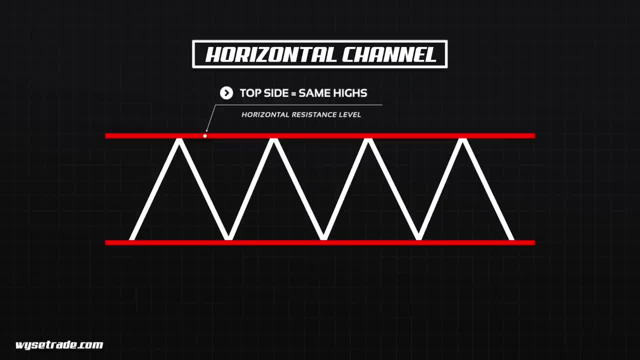 which allows for a horizontal resistance level to be placed. The bottom side of the pattern makes same lows, which also allows for a horizontal support level to be placed. The two levels are parallel to each other and in a horizontal direction. This pattern then forms: 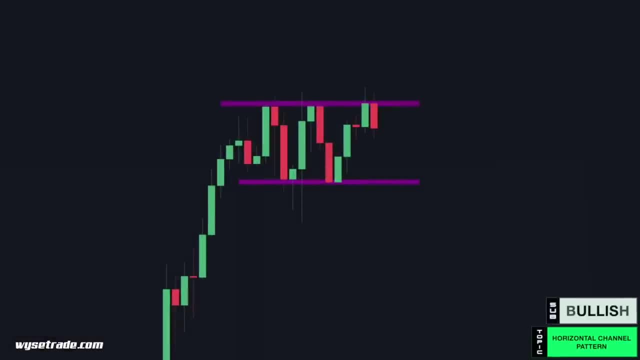 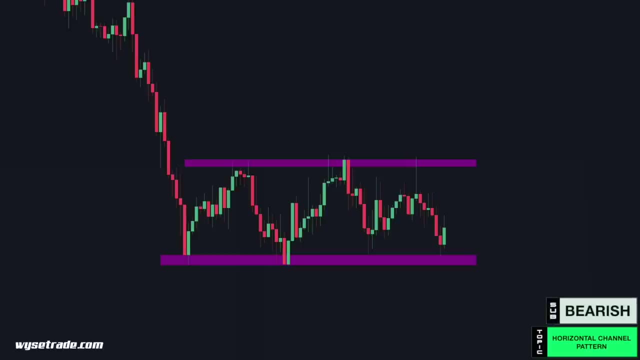 in both bullish and bearish markets. A bullish horizontal channel starts with an uptrend, followed by the pattern formation. The bearish horizontal channel starts with a downtrend, followed by the pattern formation, Also right now. if you're enjoying this video and want to. 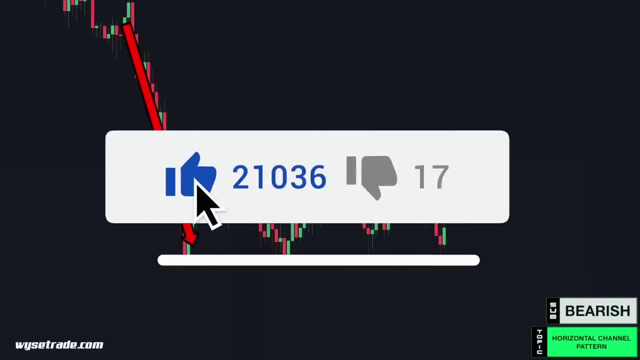 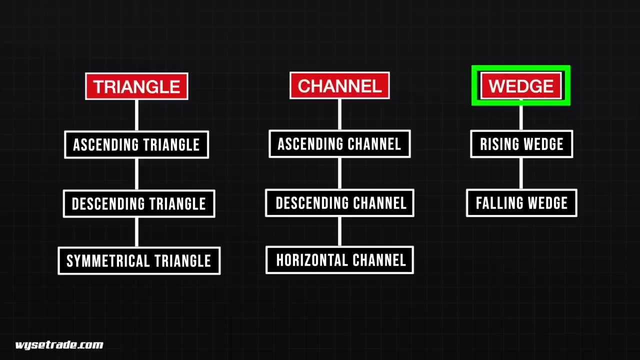 show your support. please hit the like button, as this goes a long way for us. Now moving on to the next pattern, which is the wedge pattern. So the wedge pattern has two variations. Let's start with the first, which is the rising wedge. 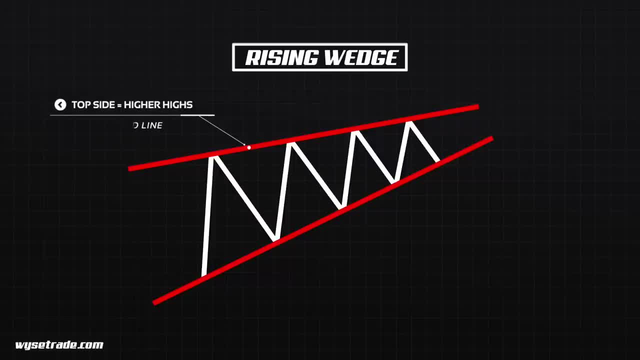 pattern. The top side of the rising wedge makes higher highs, which allows for a rising trendline to be placed. The bottom side of the pattern makes higher lows, which also allows for a rising trendline to be placed. Now, the key here is that the two trendlines are converging and are both 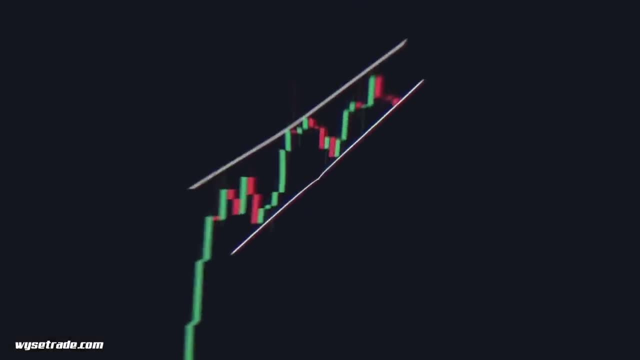 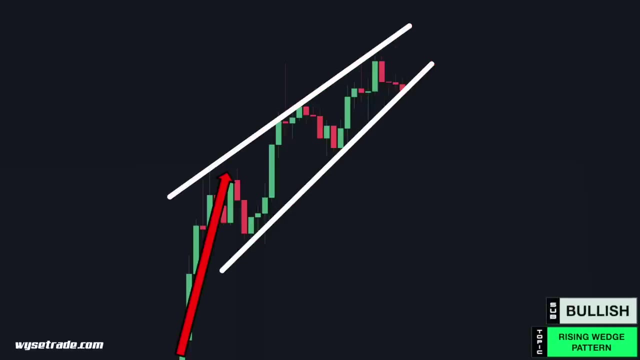 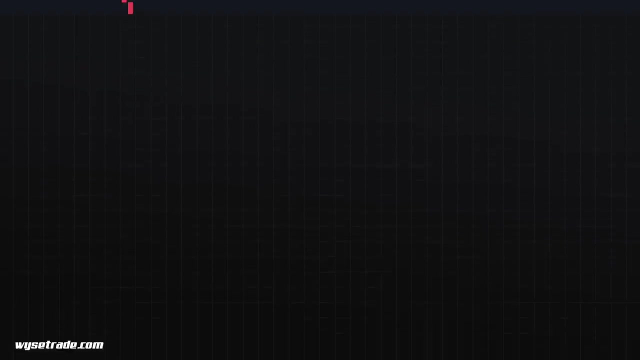 in an upwards direction. This pattern then forms in both bullish and bearish markets. A bullish rising wedge starts with an uptrend, followed by the pattern formation. A bearish rising wedge starts with a downtrend, followed by the pattern formation. So next the falling wedge pattern. The top side of the falling wedge makes lower highs. 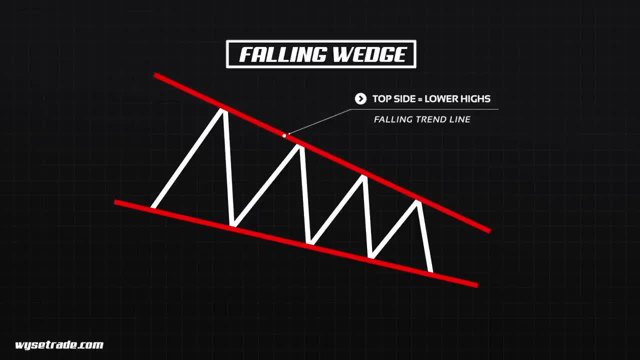 which allows for a falling trendline to be placed. The bottom side of the pattern makes lower lows, which also allows for a falling trendline to be placed. Now, the key here is that the two trendlines are converging and are both in an upwards direction. This pattern 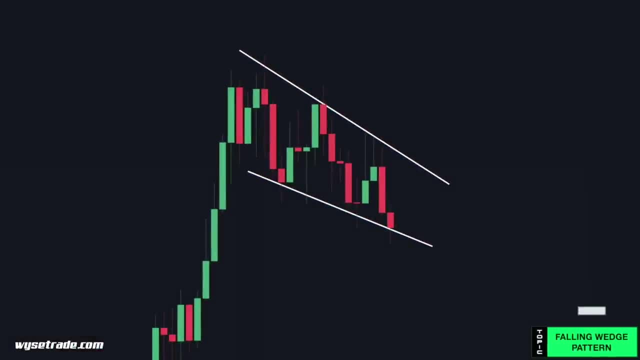 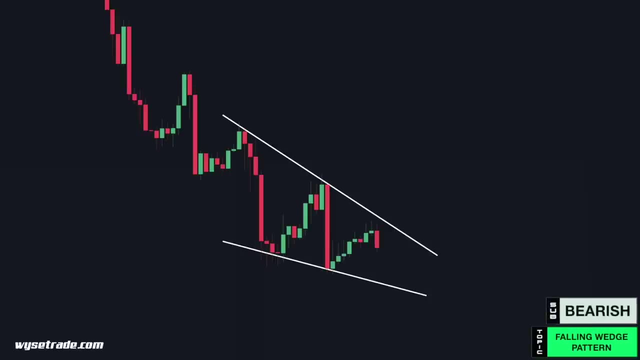 forms in together bullish and bearish markets. A bullish falling wedge starts with an uptrend, followed by the pattern formation. A bearish falling wedge starts with a downtrend, followed by the pattern formation. So, now that we have covered the three core patterns, 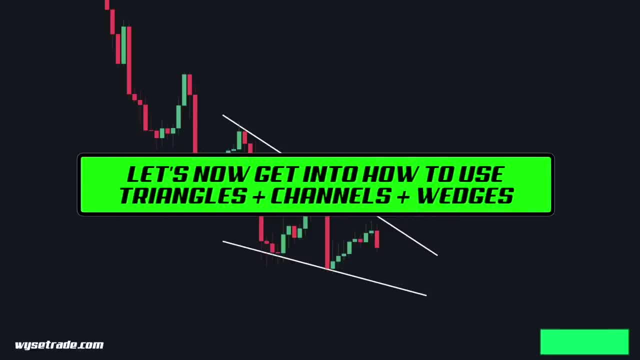 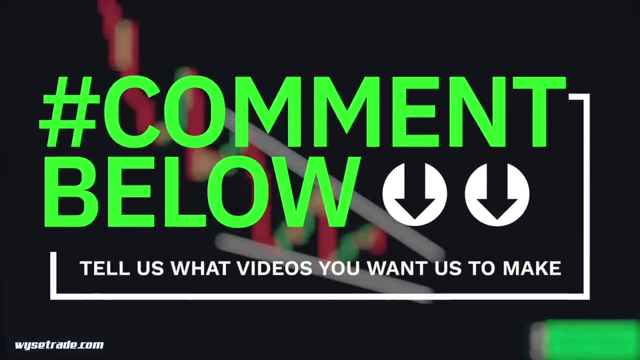 let's get into how to actually use triangles, channels and wedges as part of our strategy. If your corporate trading method is very fast, it can make some low selling best impatient reviews. Before we continue, go to the comments section right now and tell us what video topics you want us to cover next. 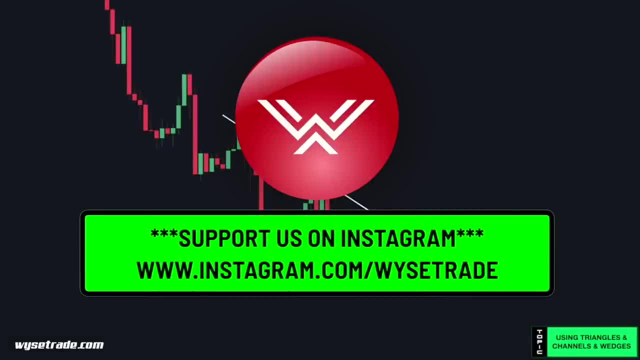 Also, to show your support, make sure you go follow us on our Instagram account at Wisetrade to stay notified about a lot of big projects we have on the way. If you are enjoying this video, please hit the like button right now as well. 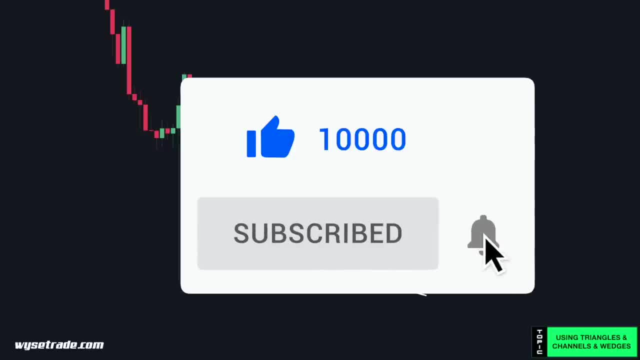 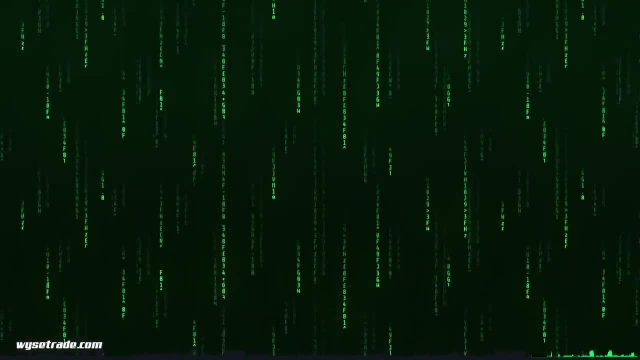 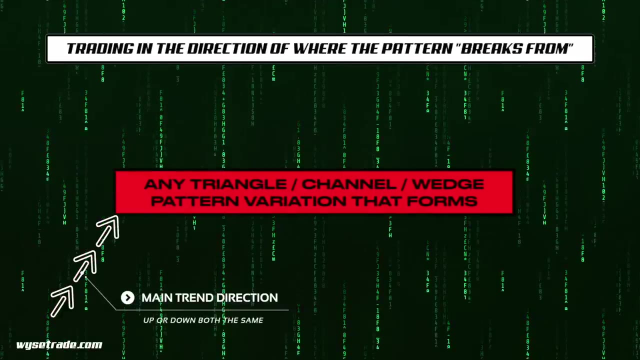 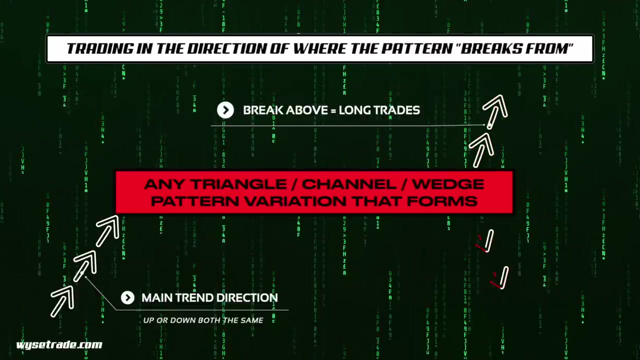 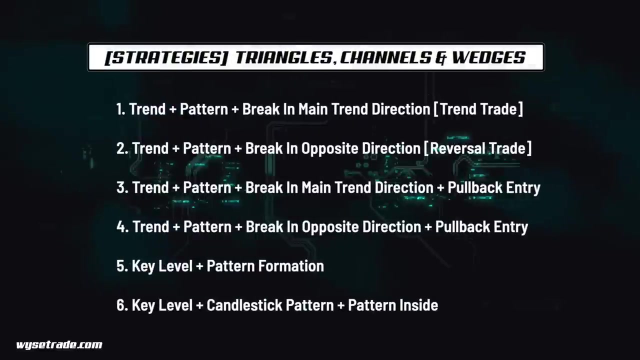 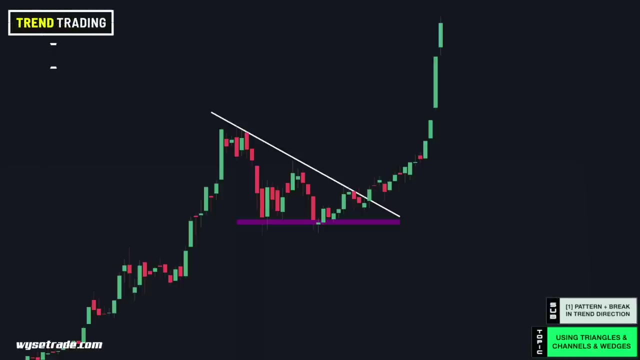 See you next time. All the strategy variations. Let's start with the first: Identifying a trend, followed by a pattern formation and then a pattern break in the main trend direction. This is a trend trading strategy. This is the Tesla stock. 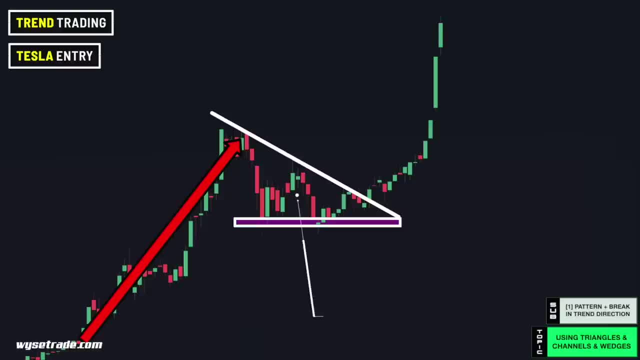 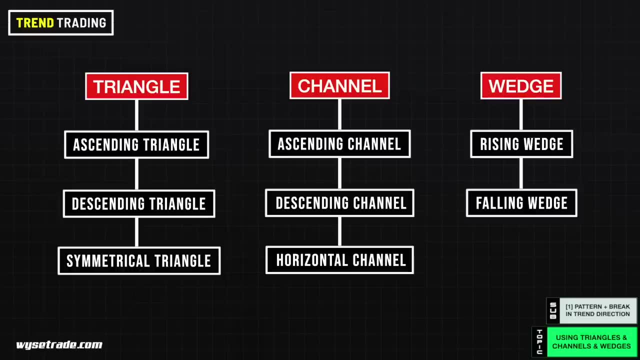 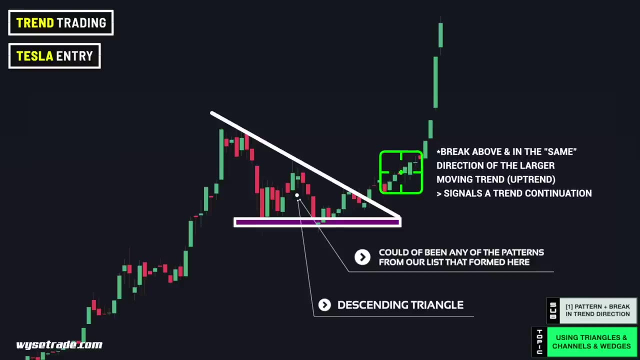 You have your moving uptrend before a descending triangle pattern forms. Again, to be clear, this here could have been any of the patterns from this list, But in this case we had the descending triangle pattern that formed. Now, if price breaks above like this, this would signal a trend continuation, as price broke in the same direction as the larger moving uptrend. 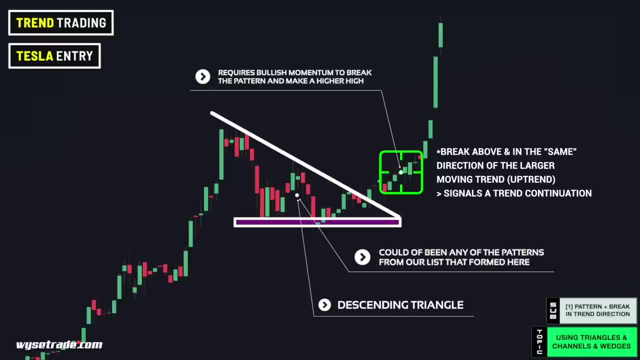 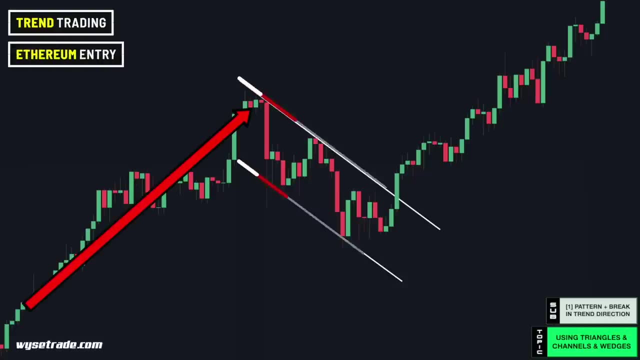 As it takes bullish momentum to break the pattern and make a higher high. You would then take long trades through the lower intraday timeframes as the trend continuation is now confirmed. Let's show this again: This is Ethereum. You had a moving uptrend before the descending channel pattern formed. 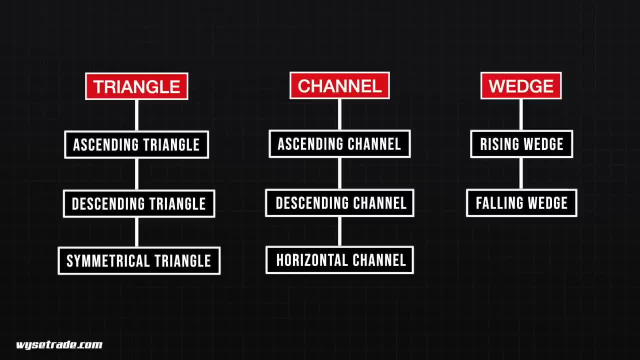 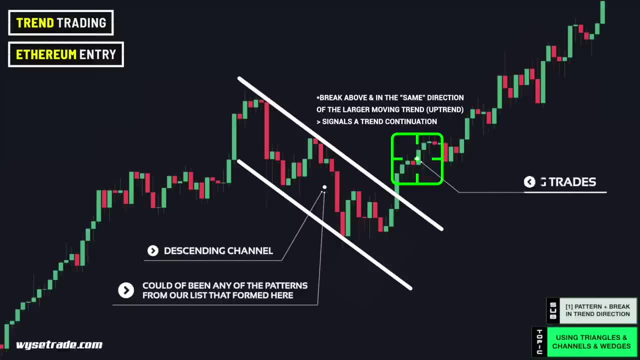 Again, it could have been any pattern from this list that formed, But in this case you had a descending channel. Now, if price breaks above like this, you would then take long trades through the lower intraday timeframes Now going the other way in a downtrend. this works the same. 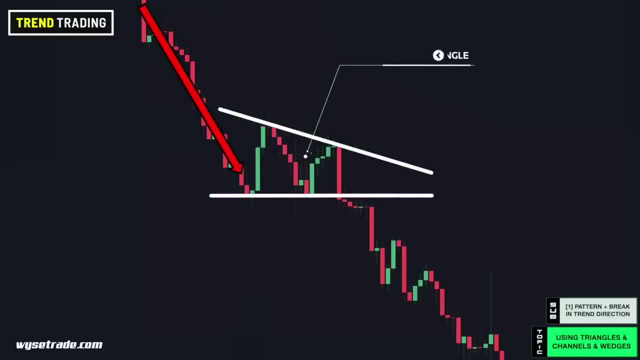 You have your moving downtrend before a descending triangle forms. Again, it could have been any pattern from this list, But in this case you had a descending triangle. Once the pattern breaks below Meaning, it breaks in the same direction of the larger moving downtrend. 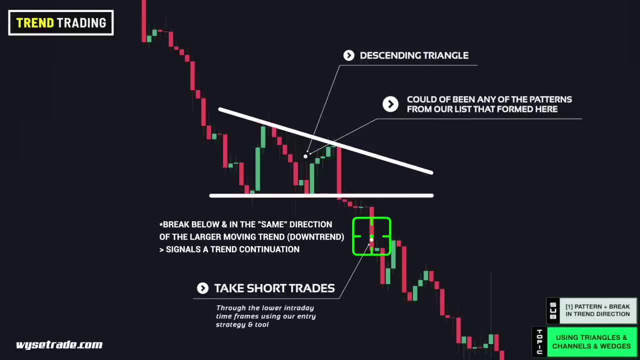 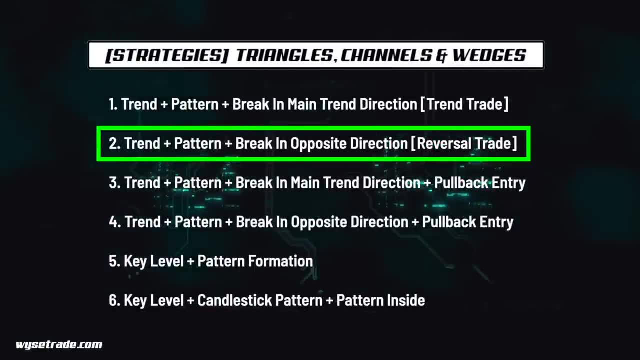 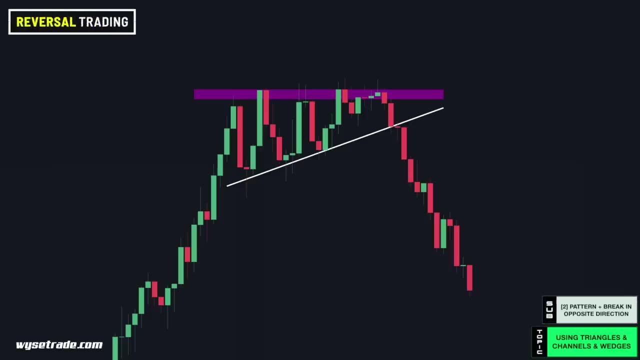 You would take trend continuation trades short. Now, moving on to the next variation, Identifying a trend followed by a pattern formation, But then a pattern break in the opposite direction of the main trend. This is a reversal trading strategy. So you first have your moving uptrend before an ascending triangle pattern forms. 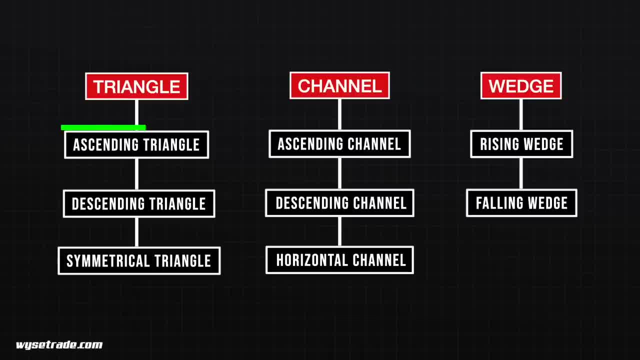 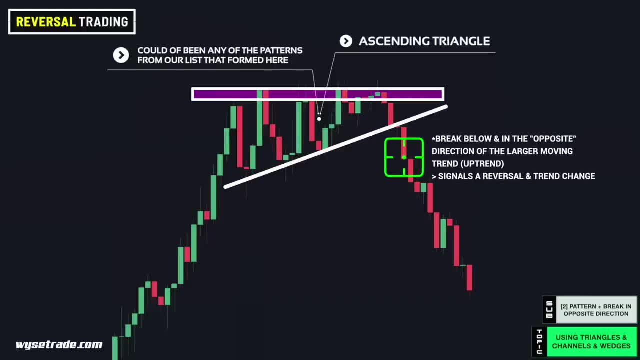 Again, it could have been any pattern from this list, But in this case You had an ascending triangle. Now the pattern breaks below and in the opposite direction of the main uptrend, Signaling a reversal and a trend change from an uptrend to a downtrend. 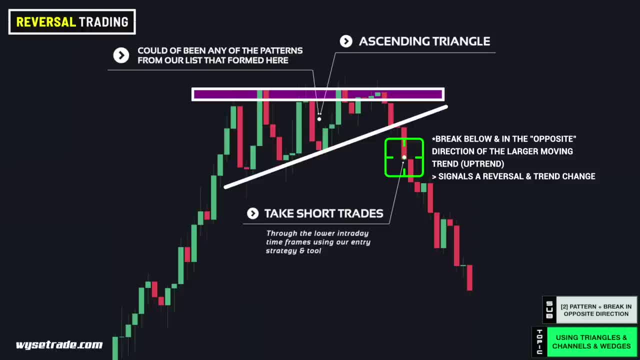 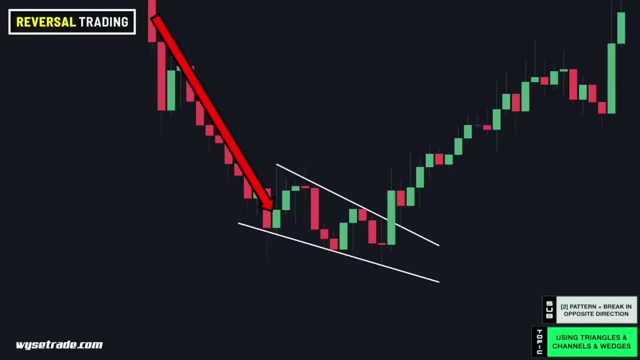 So in this case you would take trade entries short after the break below, Now going the other way in a downtrend. this works the same. You have your moving downtrend before a falling wedge pattern forms. Again. it could have been any pattern from this list. 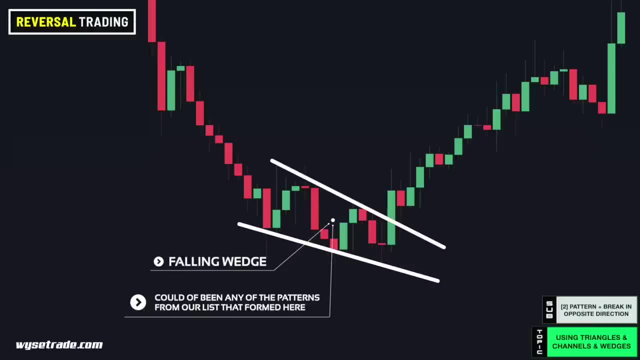 But in this case you had an ascending triangle, But in this case you had a falling wedge. Now the pattern breaks above and in the opposite direction of the main downtrend, Signaling a reversal and a trend change from a downtrend to an uptrend. 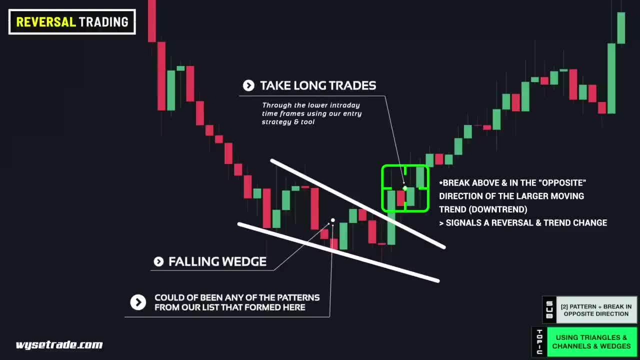 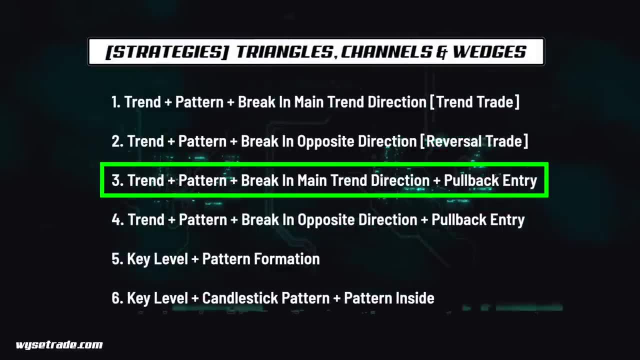 You would then take trade entries long through the lower intraday timeframes. Now, moving on to the next variation: Identifying a trend followed by a pattern formation, Followed by a break in the main trend direction, But instead of taking a breakout entry, waiting for a pullback. 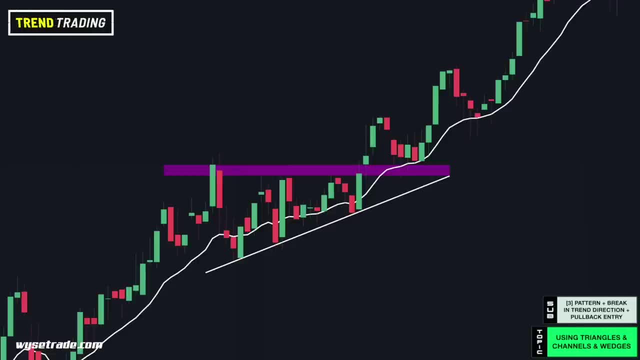 entry. This is a trend trading strategy and this is the Microsoft stock. You had your moving uptrend before an ascending triangle pattern formed Again. it could have been any pattern from this list, but in this case you had an ascending triangle. So, like we previously showed, 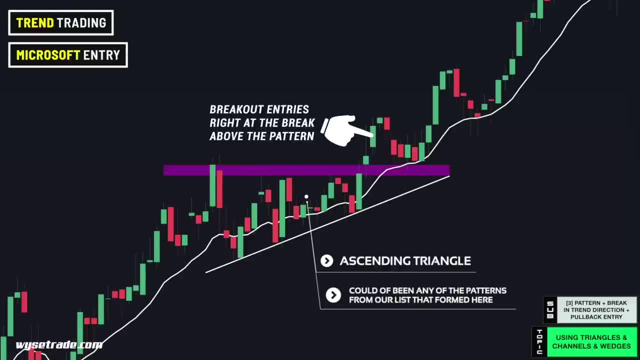 you once price breaks above. you could have taken a breakout entry long right away, But now more secure traders would wait to see if there was a pullback that occurred, which you had here through the multiple long wick candles reacting to the new support level and top side of the. 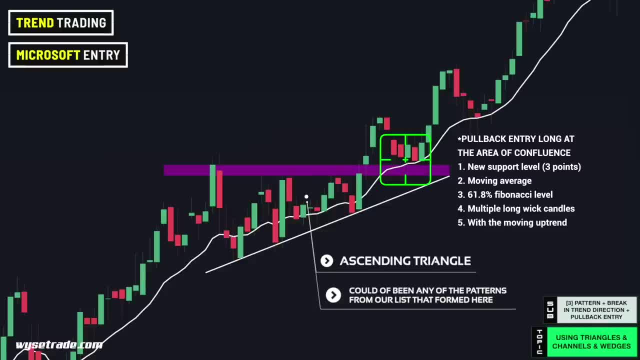 pattern and where the moving average also crossed, which creates an area of confluence. Then, once you had an intraday trend change, you would take trade entries long using our entry strategy and tool. Again, whether you trade the breakout or wait for the pullback, both work, fine It all. 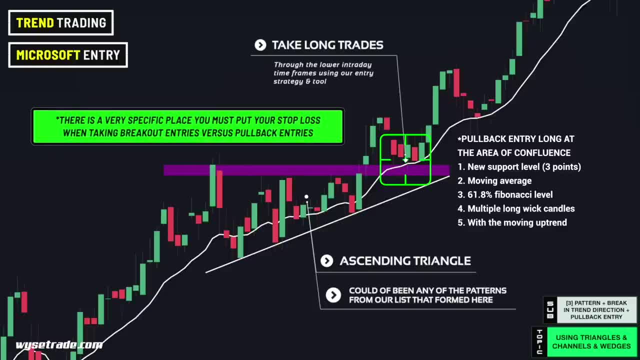 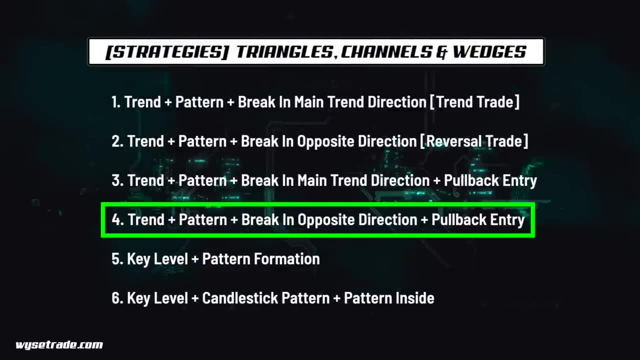 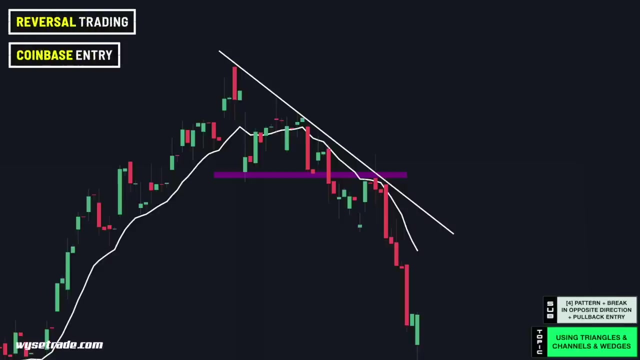 comes down to your style of trade. Now, breakout entries and pullback entries require you to place a stop. This is a reversal trading strategy. This is the Coinbase stock. You had your moving uptrend before the descending triangle pattern formed Again. it could have been any pattern from this. 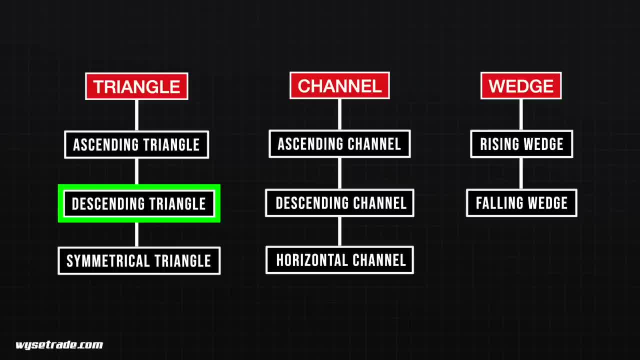 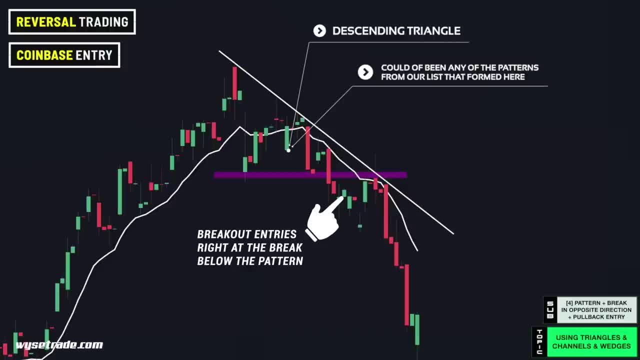 list, but in this case you had a descending triangle. So, like we previously showed you, once price breaks below this would signal a reversal from an uptrend to a downtrend and you would take breakout entries short. Now more secure traders would wait to see. 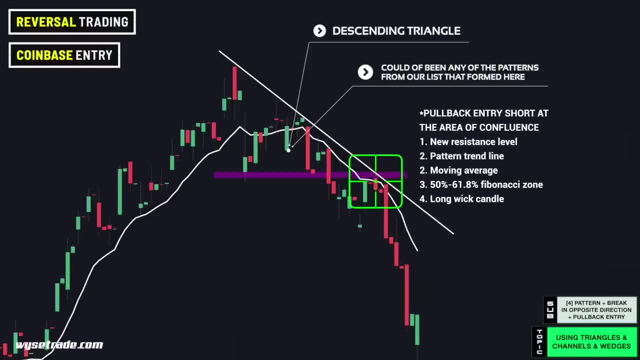 if there was a pullback that occurred, which you had here, with the long wick candle forming right at the new resistance level and bottom side of the pattern and where the pattern trendline crosses, giving you an area of confluence, Then, once you had an intraday trend change, you would 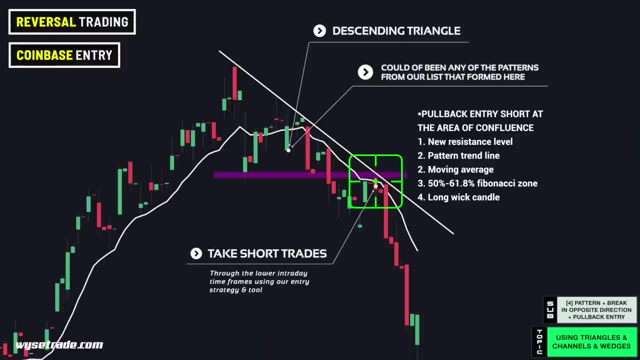 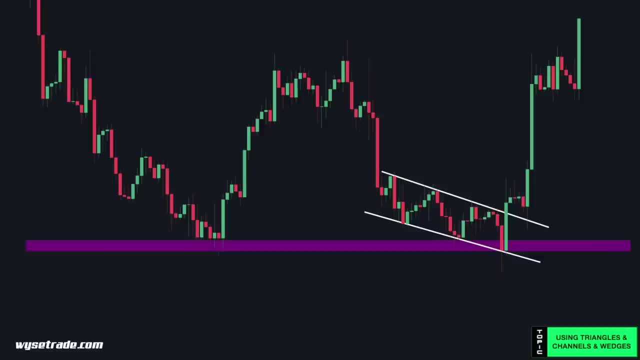 trade entries short using our entry strategy tool. Now, moving on to the next variation—a pattern forming. You first identified a key level through this reversal point. Now, as price went down, you had a descending channel pattern form right at the key level. Again, it could have been any pattern from this list, but in this case 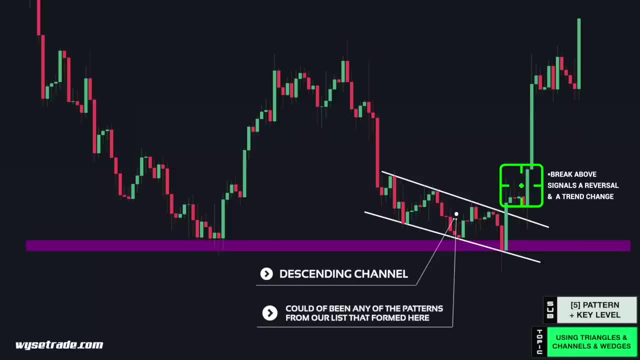 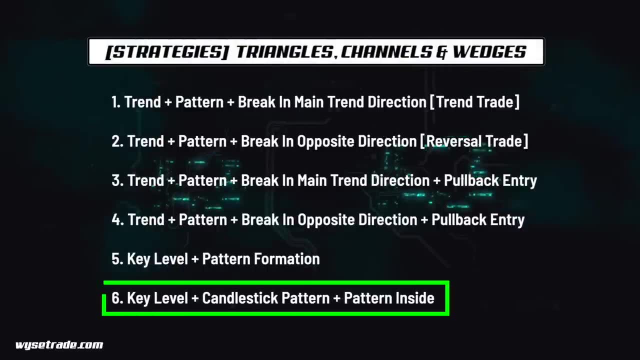 you had a descending channel form, So instead you would trade a lowờ and you would take trade entries long. Now moving on to the final variation: identifying a key level followed by a candlestick formation and then a pattern inside. 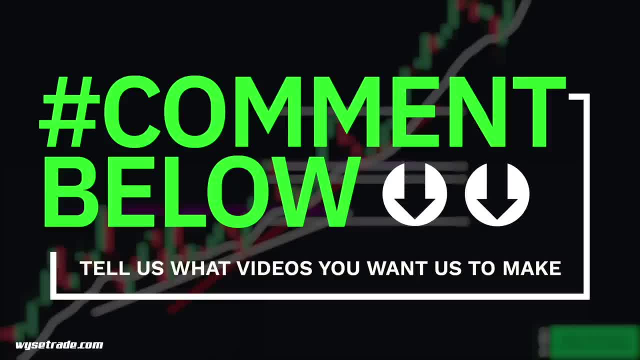 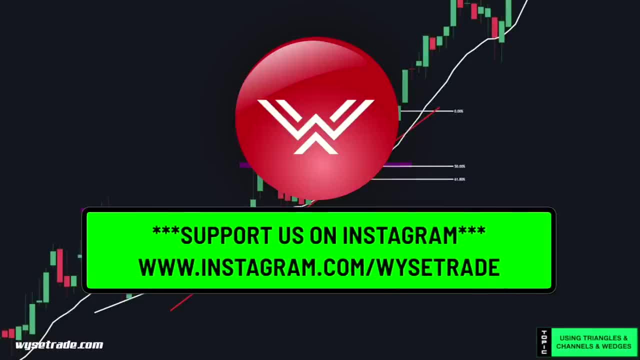 Now, before we continue, go to the comment section right now and tell us exactly what videos you want us to create next. Also, to show your support, make sure to go follow our Instagram account at wisetrade to stay notified about a lot of big projects we have on the way. 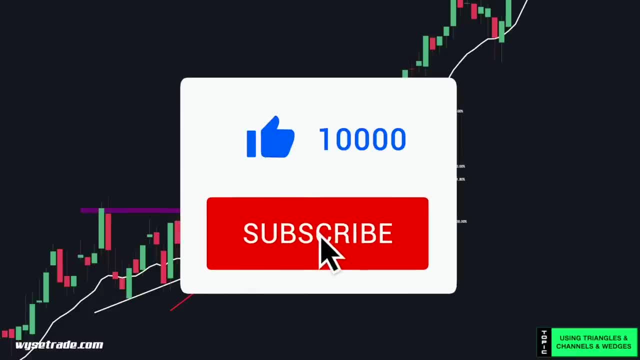 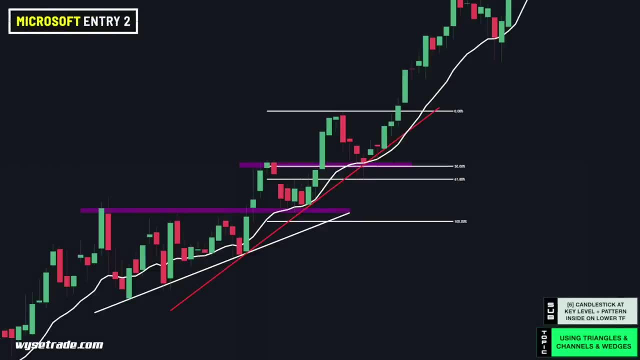 If you're enjoying this video, please hit the like button right now to show your support. So this is the Microsoft stock again. We covered this earlier, where you had your pullback entry here, but now there was a second entry using this new variation. 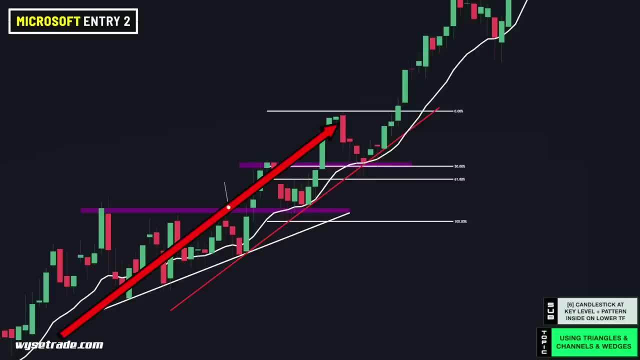 So let's list the pro traits working in your favor. First, you're trading with the moving uptrend. Next, you have the momentum from the pattern break here and the long trade entries that took place here. Then you had your area of confluence here. 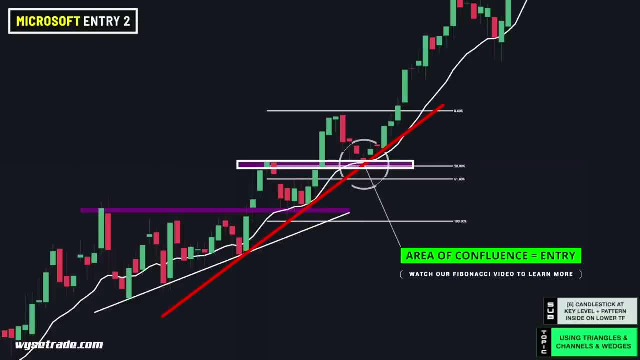 where the trend line, new support level that recently formed and moving average and fib level all crossed As price came back down to this level. you had multiple perfect, long wick candles reacting to the area of confluence. So after you had the candles reacting, 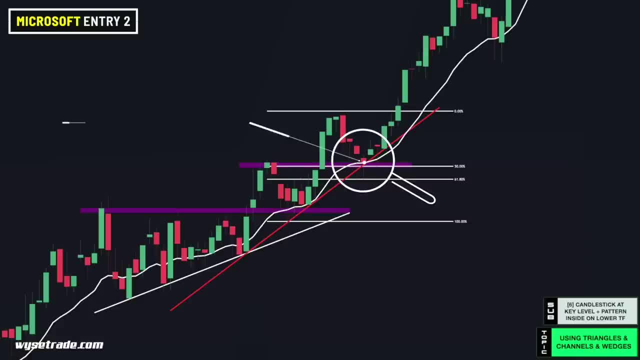 to the area of confluence. you need to look inside of the candles and inside out inside of this area to find price action that signals a trend change from a downtrend to an uptrend, Because, even though this is a strong moving uptrend here, 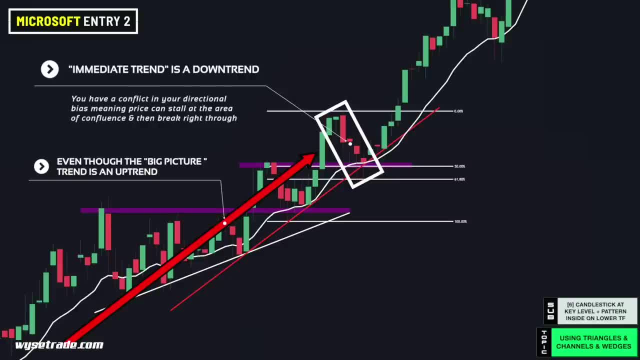 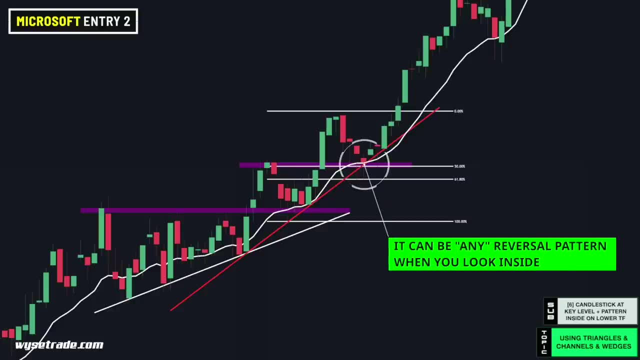 this here is a short-term downtrend, meaning price can stall at the area of confluence and then break right through, triggering a larger trend change. Now a key note: when you look inside of this area, it doesn't have to be a wedge triangle or channel. 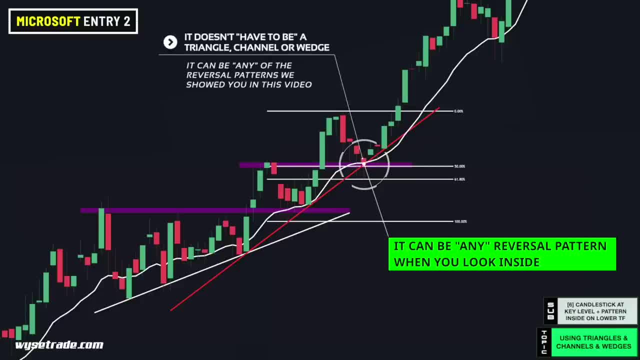 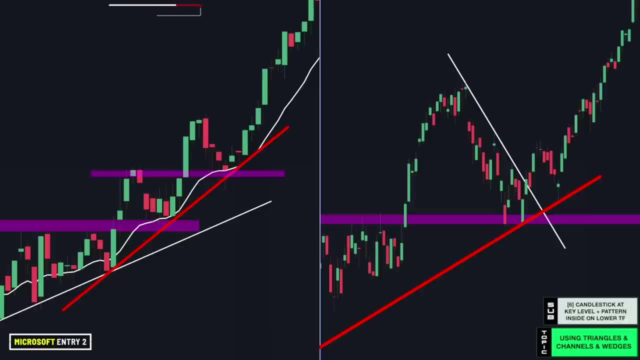 It can be any of the previous patterns we showed you in this video. All the reversal patterns work the same, So let's pull up the daily timeframe and put it beside this one. The chart on the left is the Microsoft weekly timeframe we just looked at. 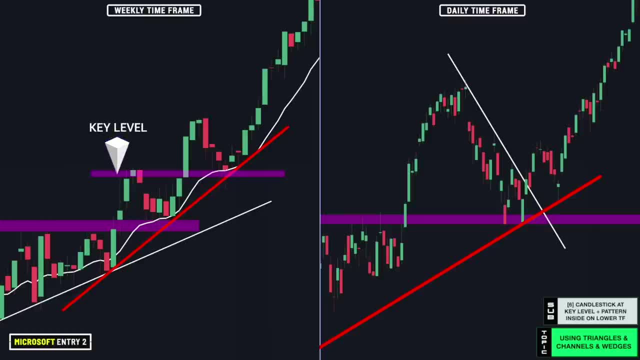 and on the right is the daily timeframe. This key level here is this same key level here. This area of confluence here and where the candlesticks formed, is this same area. here, Again, we're looking for any form of price action. 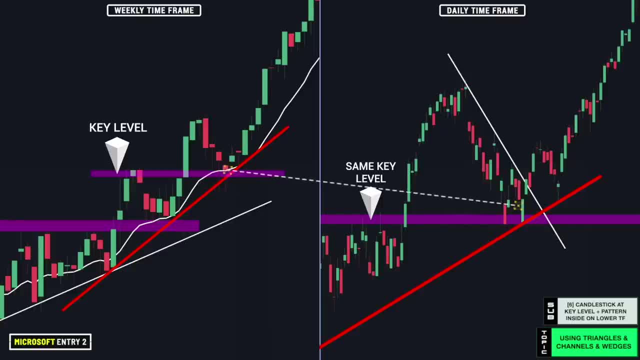 that signals a trend change from a downtrend to an uptrend. So what we had in this case here was a perfect descending triangle pattern that formed right up to this point, Right at the area of confluence from the weekly. Then, once price breaks above and makes the higher high, 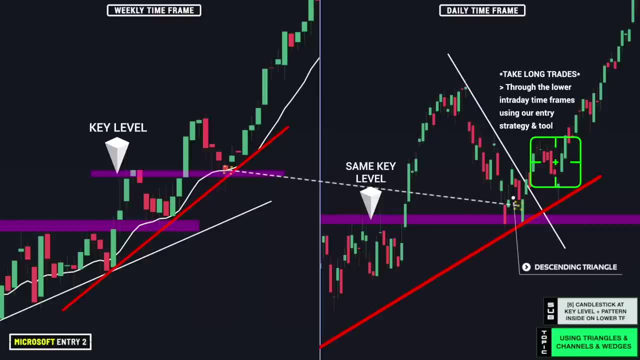 the trend change is confirmed from a downtrend to an uptrend. Now here's a very key point. Notice how price didn't go straight up after the break and pulls back slightly before actually taking off upwards. And this is why you need the two most important parts. 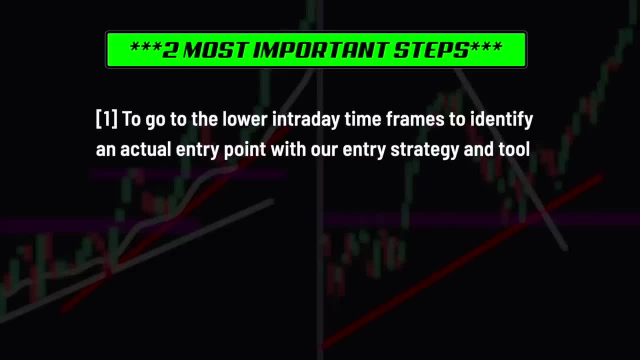 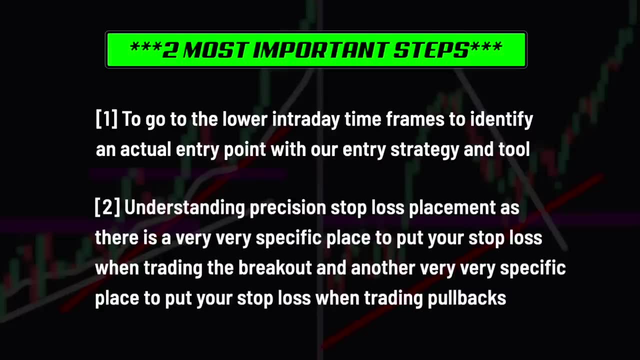 One, to go to the lower intraday timeframes to identify an actual entry point after the break using our entry strategy and tool. And two, understanding precision stop-loss placement, as there is a very specific place to put your stop-loss when trading the breakout.